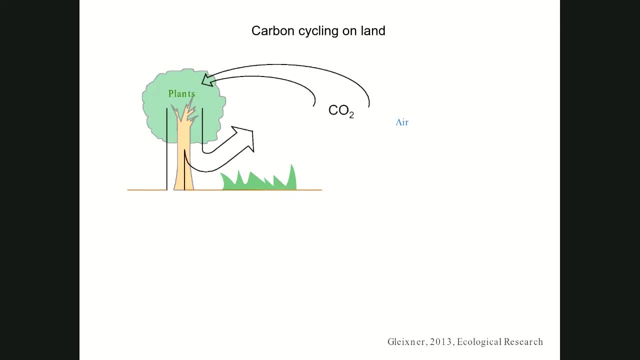 We know from our textbook biology knowledge that plants fix carbon dioxide using energy from sunlight, and once they fix carbon, the plant organic matter is then returned to the environment below ground in the form of leaf or root litter, but also in the form of root. 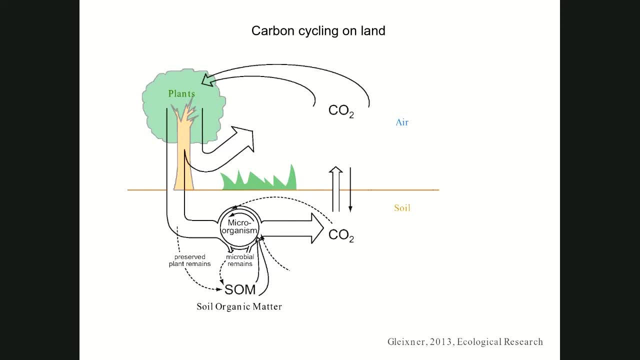 exudates, which are nice juicy substances that plants secrete into the soil, But below ground microbes take the center stage, So they're at the center of below ground carbon cycling, And what the microorganisms do is that they break down the organic matter and they convert. 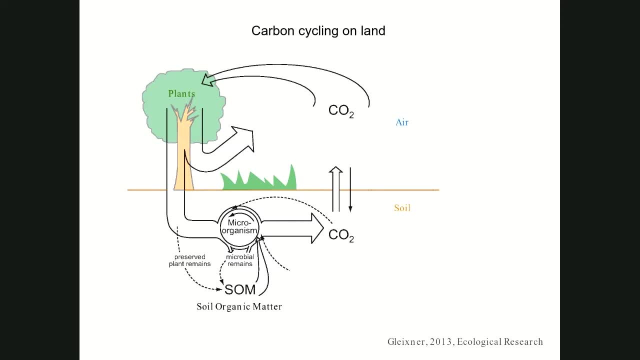 it into microbial biomass, And some of the new research suggests that most of the soil organic matter is not organic. The organic matter which is the soil humus, is mostly remains of microbial dead matter, and it's not plant remains, So in that sense, microorganisms are contributing massively to below ground carbon cycling. 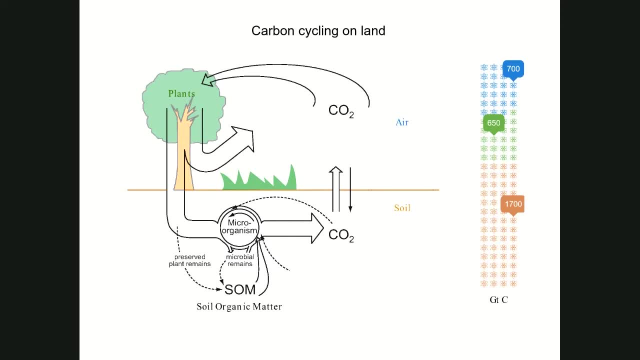 And in terms of the carbon budget, if you look at how much of carbon exists in the soils below, So you can see here this is gigatons of carbon. It's more than the amount of carbon in all the plants on the earth and the atmosphere put. 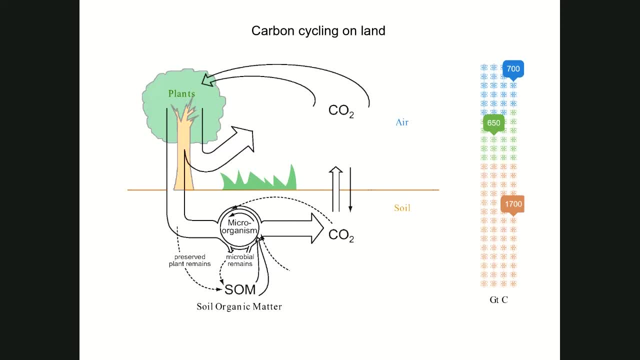 together And this shows you how big the soil carbon pool is. But in addition to that, it's also a very dynamic pool, So there are fluxes that can alter the balance between the atmosphere. I'm missing this point And because of this reason, it's very key to study the below-ground carbon cycling, because in future, this balance can be affected in a big way. 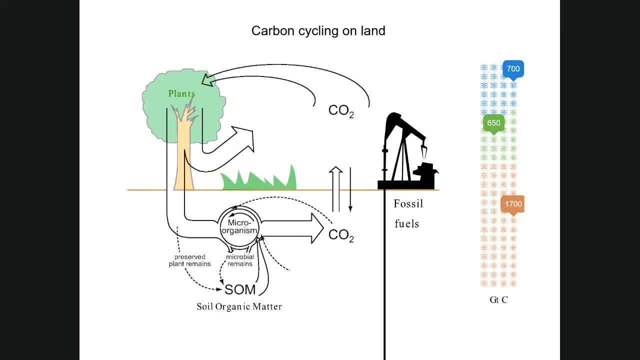 And we know that. what fossil fuels are? they're carbon, basically in the deep earth, And human activities are leading to an increase in CO2 in the atmosphere which is causing an imbalance in the environment. So global warming is leading to climate change and it's affecting the whole carbon cycle. 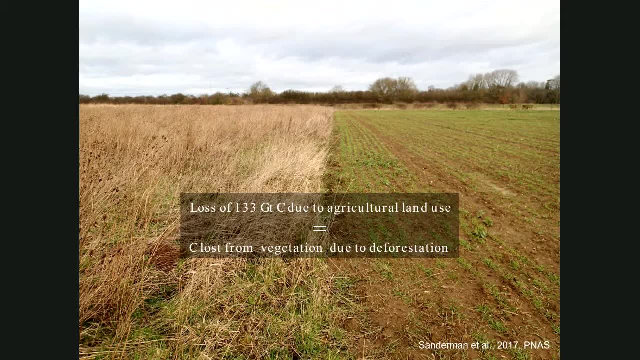 But in terms of agriculture, historical land use, there are some estimates that about 133 gigatons of carbon was lost due to agricultural land use, And this is since agriculture began as a practice. This is equal to the amount of carbon that's being lost through deforestation. 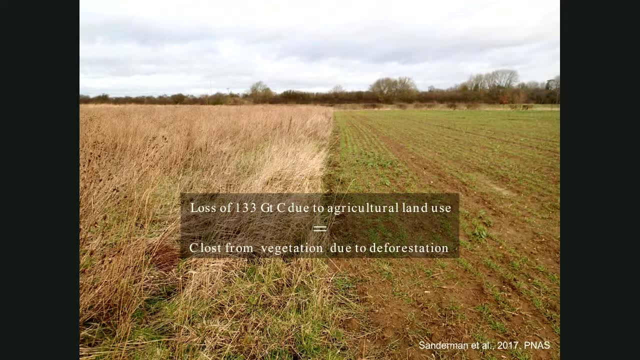 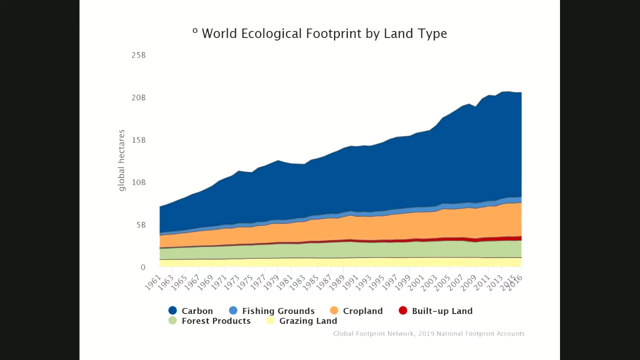 So it's as big a loss And if we look at this in terms of the budgets, you can see that it's a massive amount. And it's not just a legacy of carbon, It's a legacy of the past, But in the past like in the past, distance like contemporary history, since this data from the Global Footprint Network is from the 60s. 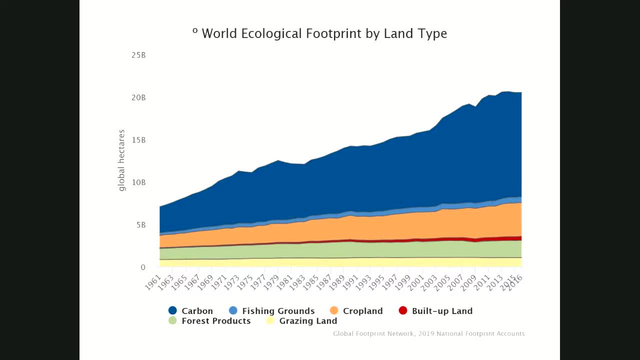 suggests a rapid increase in the carbon footprint coming from cropland and using land. So agricultural practices are contributing to carbon As in addition to the fossil fuels, which are obviously a massive contribution to the carbon footprint across the across the world. So this suggests that land use change is also an important factor which needs to be considered while planning strategies for climate change mitigation. 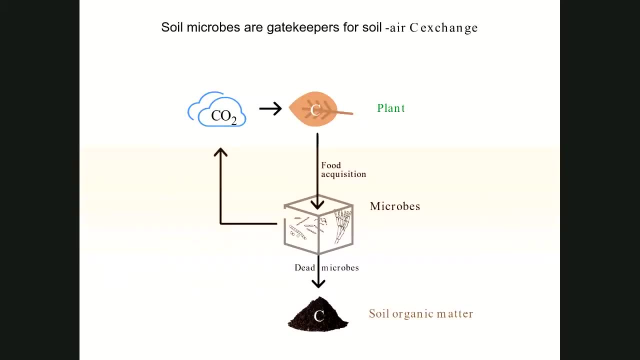 And how do microbes come into picture? Soil microbes- they are gatekeepers of the soil atmosphere. carbon exchange, So plants fix carbon and then much of the plant matter is is food for microorganisms. Once they have access to this, they they, they use it to grow or they use it for other maintenance purposes. 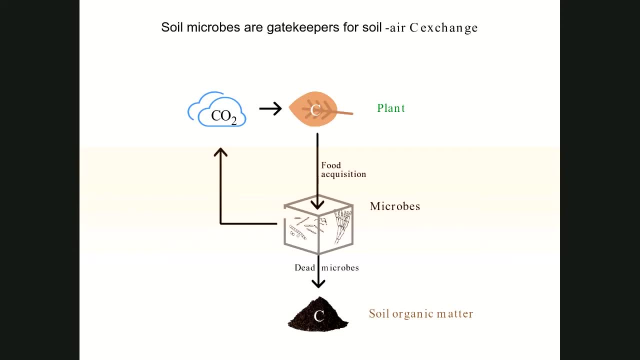 Like: if there is there is stress in the environment, they use it to alleviate that stress. If there are not, mean that if there's not much food in the environment. So for them- for hydrotrophic microbes, it's mostly organic matter that comes from plants- is the resources. 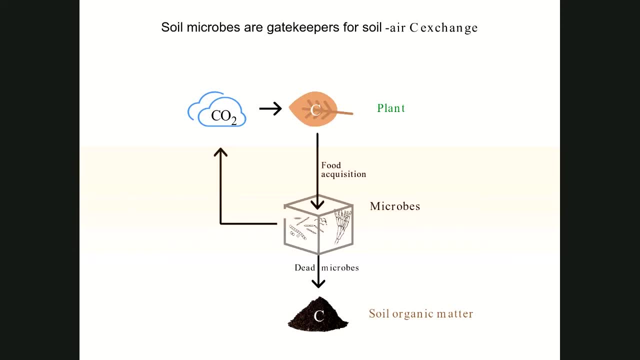 If there are limited resources, then they have to produce a lot of extracellular enzymes or to discover resources, They have to be mobile. So in order to reach the resource, So all these, all these activities then lead to, leads to lower growth because because there is limited supply of resources. 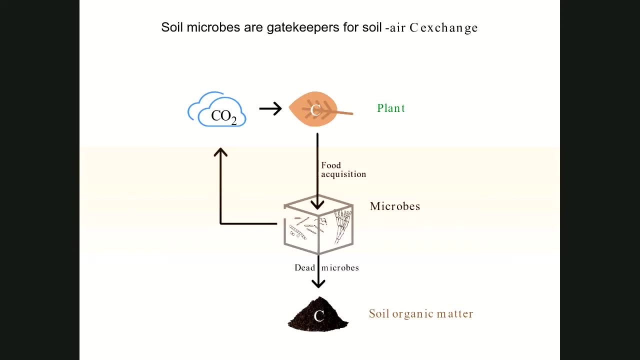 And when there are resources, they have to allocate either for one strategy or the other, So it's at the expense of the other, which means that there are trade offs in some of these strategies And once microbes grow and then they die, so it's a rapid turnover. 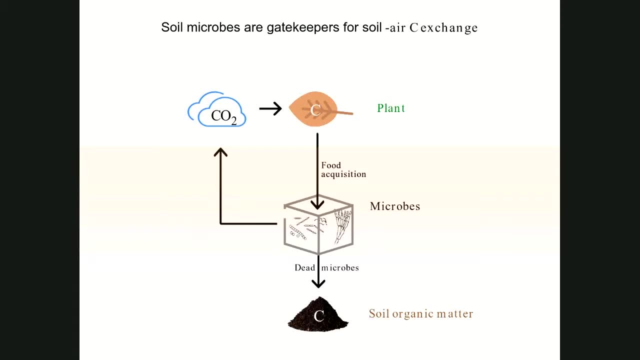 Microbial life is is is very short. The dead micro microbial biomass, which we often called necromass, then associates itself with the minerals in the soil and that for soil organic matter, And some of the newer research in the last decade or so suggests that most of the soil organic matter is a result of this necromass interaction with the mineral fraction in soils. 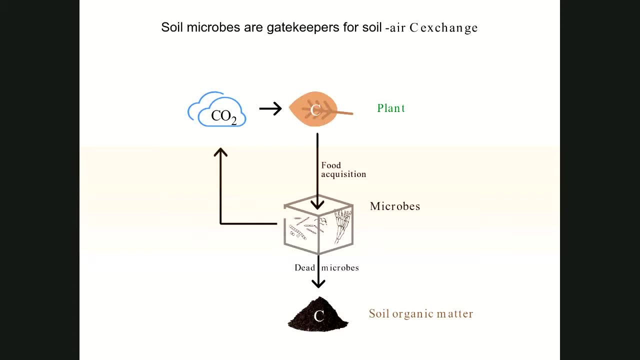 So what my research does is it looks at some of these important traits Of microbes And we we have these huge data sets of microbes Based on newer sequencing technologies, which, which is allowing us to improve our understanding of microbial processes, is a lot of information. 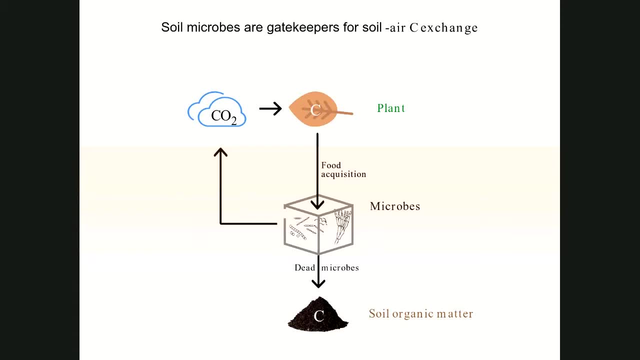 So my trait based approach is trying to distill That information so that we we make meaningful linkages to environmental processes like soil carbon sequestration. So to give an example of how this trait based approach has been applied, This is a study that was done during my postdoc at the Center for Ecology and Hydrology in Wallingford in Oxfordshire. 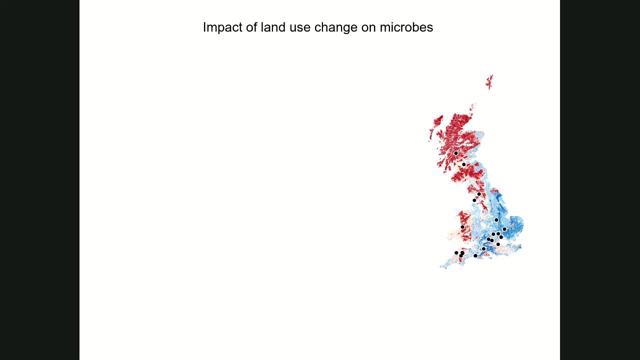 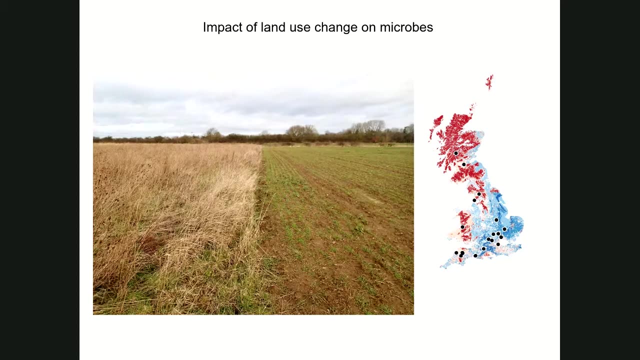 And here we sampled soils from the UK at 28 sites and each site had a local land use contrast: So often it was an over the fence or next to each other. contrast of a pristine habitat, mostly an undisturbed grassland, or or or a grassland which has been. 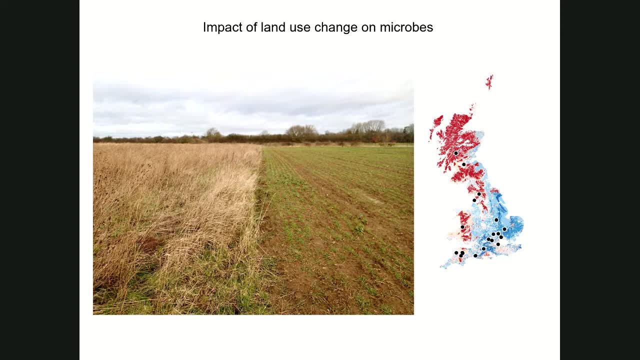 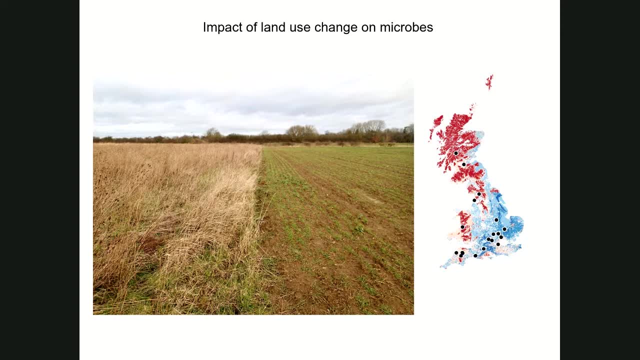 This local contrast meant that we could really understand the the impact the land management on the microbial processes and the soil carbon processes, that we could really understand the impact of the land management on the microbial processes and the soil carbon processes, um while keeping the climate and the parent material same. so that that meant that these 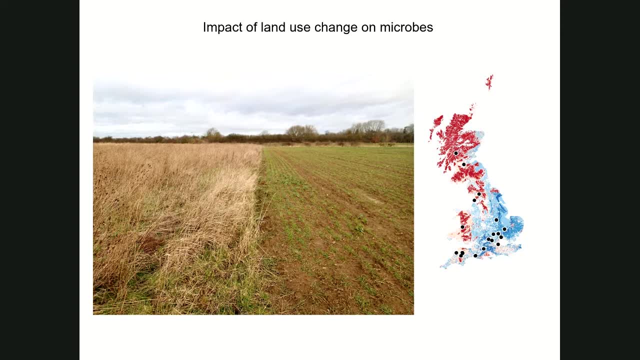 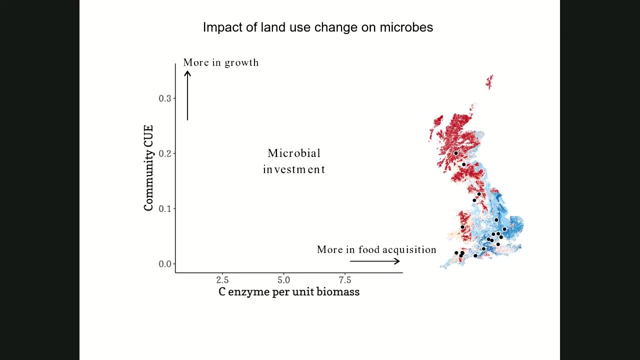 paired contrasts were really good um experimental treatments for us to look at the microbial responses to land land management. what we measured here was um community carbon use efficiency which, see you, each is on the y-axis here, um so each of the soil was used for for these measurements. 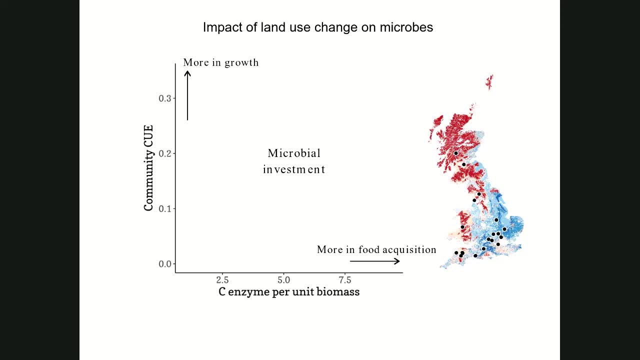 um and community carbon use efficiency is the growth yield of the community. so what we do here is we give the microbial community a substrate that's labeled with the heavy isotope of carbon, so that's 13 carbon, and and then we track that 13c into the microbial DNA, into the microbially respired carbon dioxide. 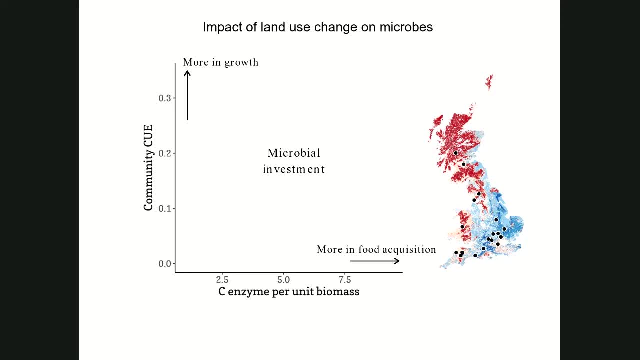 and this allows us to understand the microbial partitioning of carbon into growth versus maintenance respiration. so so if microbes are more efficient, the carbon use efficiency is higher. so that means are allocating more into growth processes. and we also measured the enzyme investment. so here we measured the extracellular enzyme production and this was per unit biomass and we measured a couple. 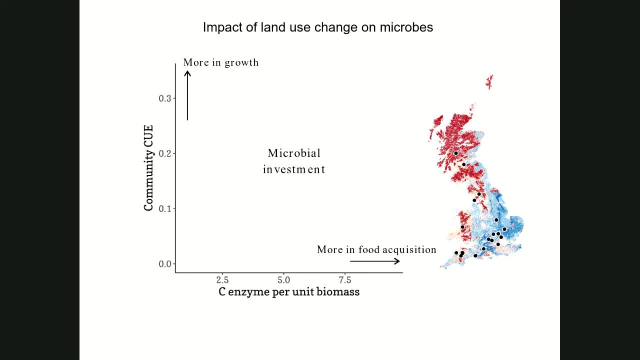 of enzymes using the fluorometric assays. so what we do is we add a substrate for a particular enzyme and if there is more of that enzyme produced by the community, then more of that substrate is broken down and you get higher fluorescence. so if we have higher enzyme production in terms 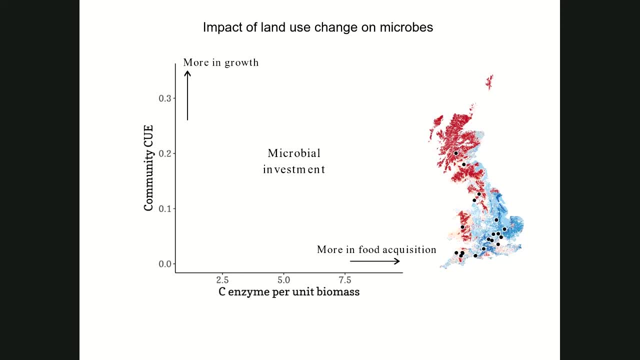 of potential activity. then we see a higher enzyme activity per unit biomass, and that means microbes are investing more into food acquisition. so how? how does the result look here? so we have a. we have a nice distribution of all our samples taken from all these sites with paired land use contrasts, and there is not a linear relationship. 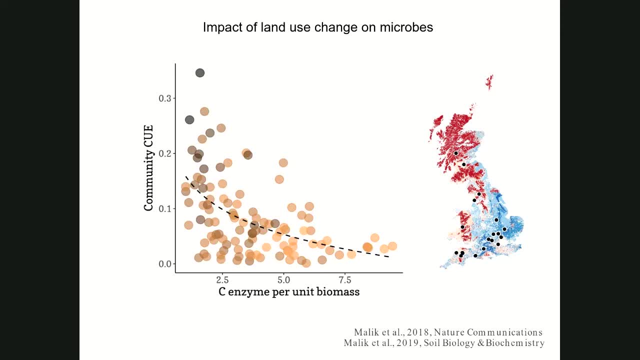 but there is a somewhat logarithmic relationship here and and then, as you can see here, that increasing enzyme investment means decreasing carbon use efficiency. in other words, if microbes are investing more into resource acquisition, that means they are not growing that well, that they are not investing that much into biosynthesis. 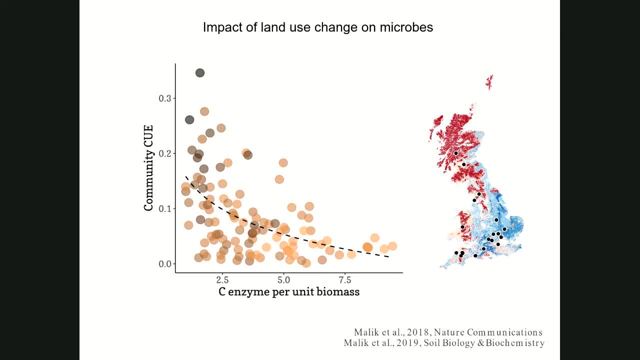 and growth and, as you can see here, i've labeled the points with this. they're shaded and that is actually the soil: organic carbon concentration. so what we see here is that the darker shade are the are the soils coming from more pristine habitats and the the lighter are coming from more um intensive habitats, so the 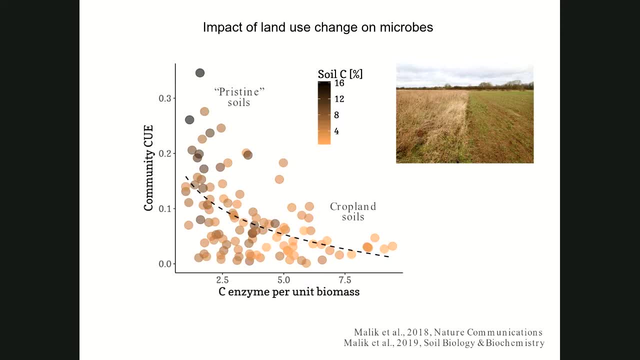 agricultural cropland soils, as you can see here that they are investing a lot into. they're investing a lot into resource acquisition, whereas there is more growth happening in the more pristine soils- I say pristine because they are not really pristine, we hardly have that- completely natural habitats here, so they are less intensive land, land use soils. so we see 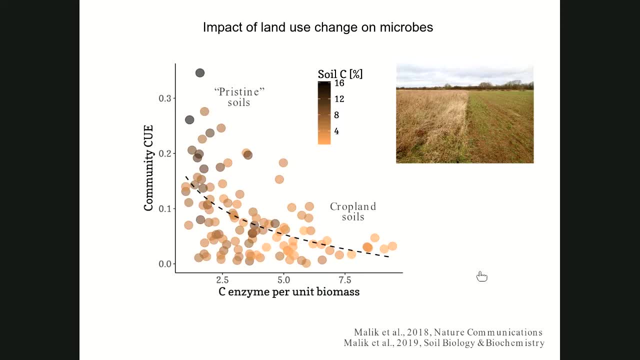 here clearly that in in the more natural habitats the microbial communities have good amount of resources available to them, because here we are not taking away the plant material for food production, for example, or in grazed and grazed land use. it's taken away by animals, livestock, but the microbes have. 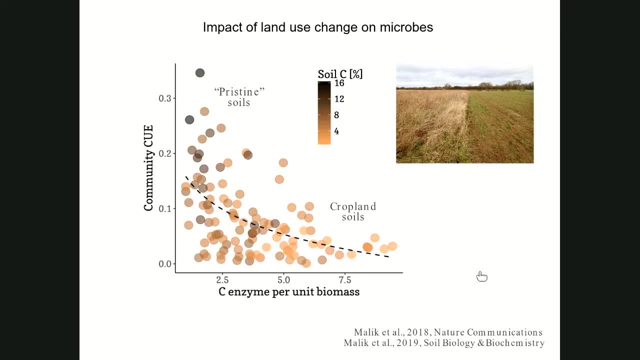 enough food there, so they're investing. they don't need to produce a lot of extracellular enzymes, they just need some transporters to suck those easily available resources, substrates- into the cell and therefore they grow really well, and this is then seen in terms of growth yield, and when you have a higher growth yield, it translates into higher 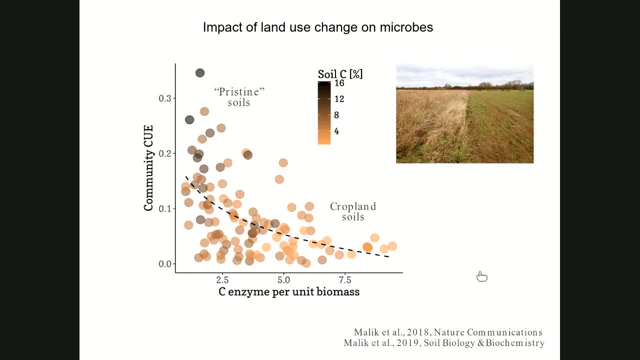 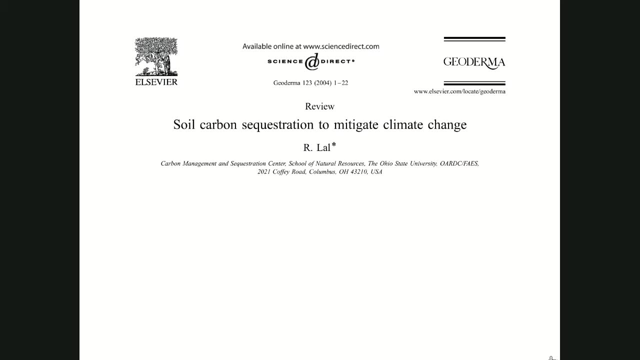 cup higher soil carbon accumulation, storage and sequestration, so the idea of using soil carbon sequestration to mitigate climate change is not that new. this was a review by Rattanlal in 2004, where some of these carbon management strategies were released by the US and other countries, and so these were used in the process of 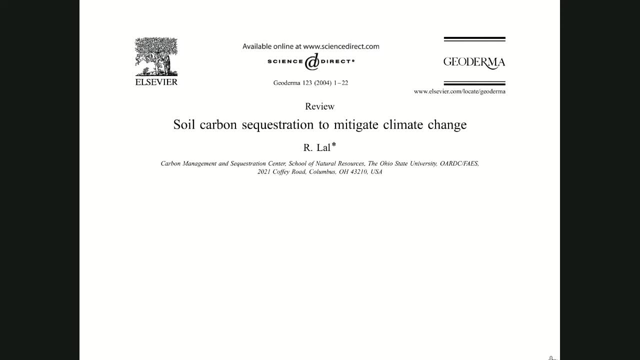 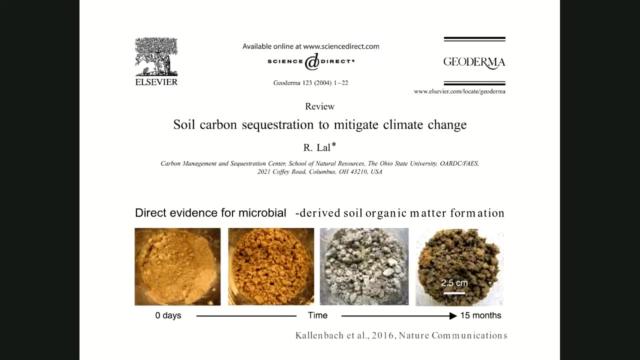 climate change management and the way of implementation. those were some of the ways of implementation of these in the process of were first coined, But then, in the last decade or so, we have improved our understanding of soil carbon cycling processes and we now know that microbial-derived organic matter 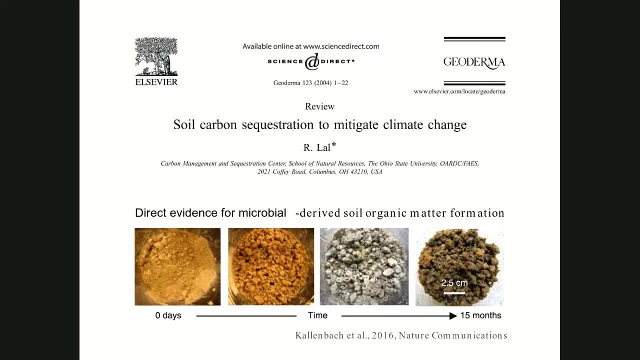 formation is a very important process in soils. So this paper here by Kallenbach et al in 2006 is a very good demonstration of microbes producing soil organic matter. So they used soil which were carbon and microbe-free and then they added a microbial community to that. 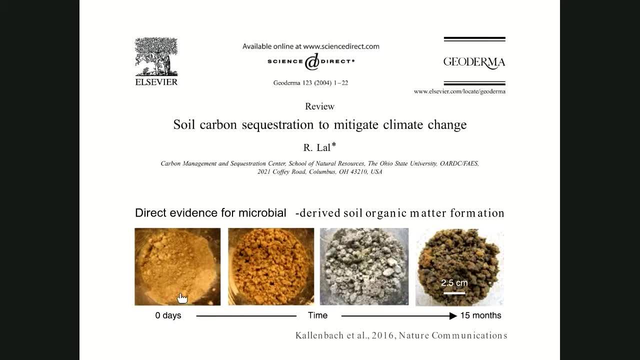 to these soils And they also added some dissolved organic matter as inputs of organic matter- Organic matter for the microbial communities- And they tracked these soils in the lab for about 15 months and they could see build-up organic matter So soils being made in the 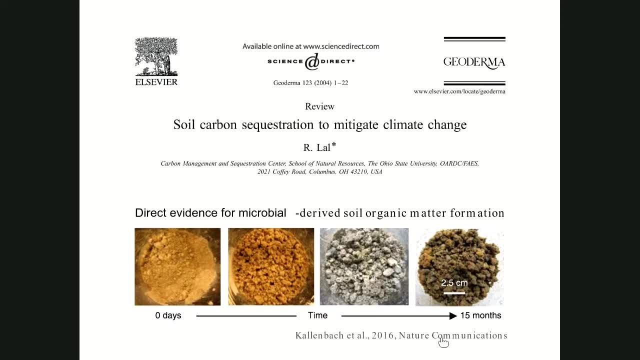 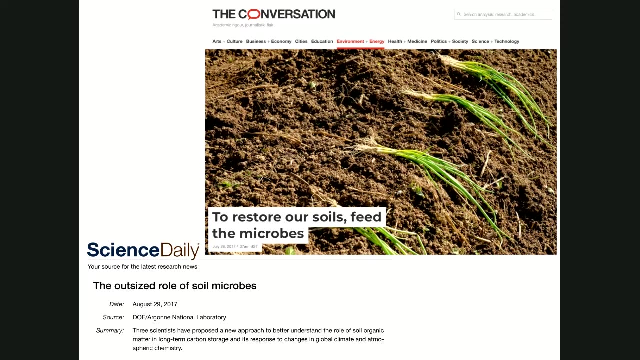 laboratory. This is a classical example of how microbes are contributing to soil organic matter formation, and this is mostly through growth and death cycles. So since then there's been an increasing realization, not just among the scientific community, but this has been taken up by a lot of stakeholders, policy makers and even 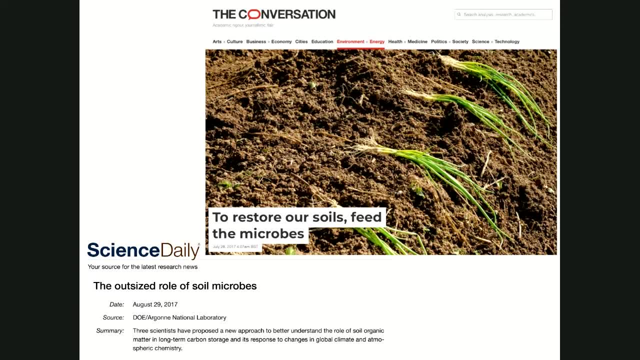 a lot of farmers now realize the importance of microbes in soil, not just in terms of carbon sequestration, but improving soil health as a whole. If there is more carbon storage in soil, it also improves soil quality. So this is a very good example of how we can. 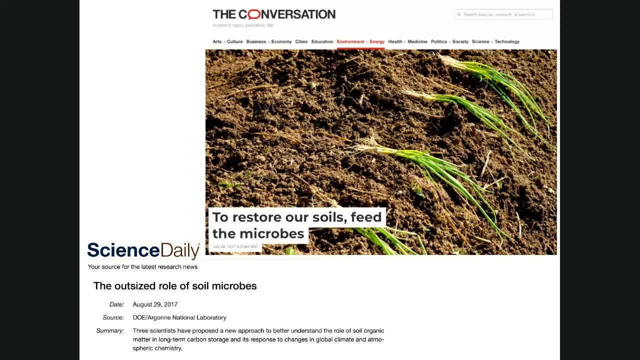 improve soil health as a whole. If there is more carbon storage in soil, it also improves soil quality. There are a lot of awesome whether we're talking about, So you can really see how this all happens inナ Organic Matters domain. What about the soil fuels for this? 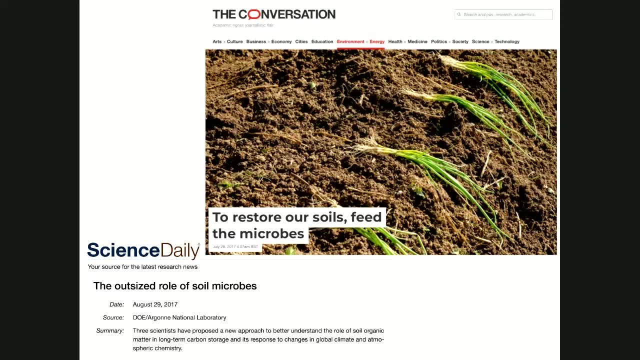 We don't graph drama, We're debating how we do it. So you can make a map of that land. it's several lines of data. What about the soil costs? There's not a lot of crushing percentages over that. this is under a budget. 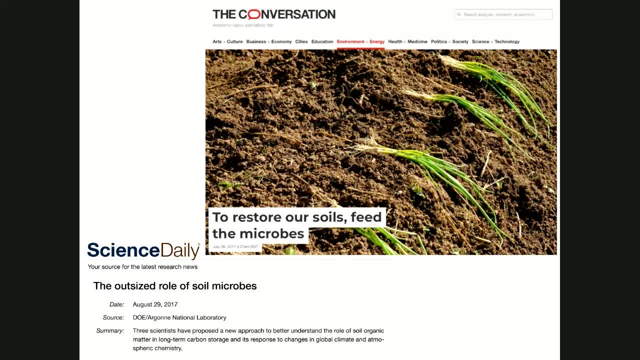 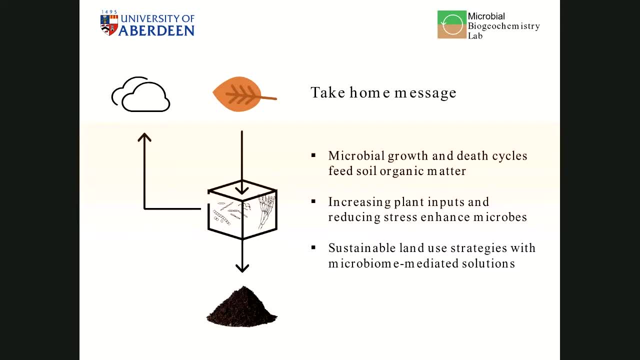 There's due process So you can calculate that. So there could be littleõ. So perhaps in a concept permitting See how we might be comparing soil oil strategies so that if there's not that much, there is an center ofOb And they really need to understand microbial processes and how they are shaped by resource. 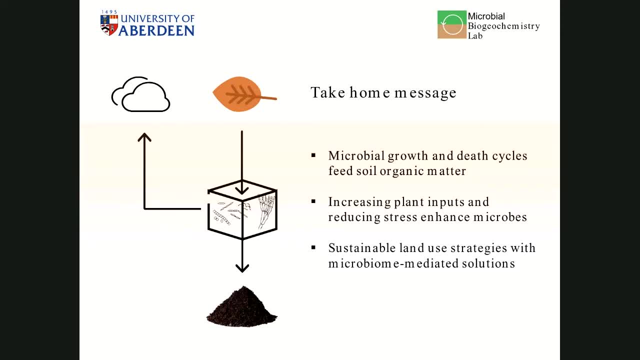 inputs, but also abiotic stresses that are arising because of changing climate, with increased incidences of droughts and floods and extreme events. So it's really important to understand these processes that are leading to formation of soil organic matter. But from what we know so far, it's very likely that increasing plant inputs and reducing 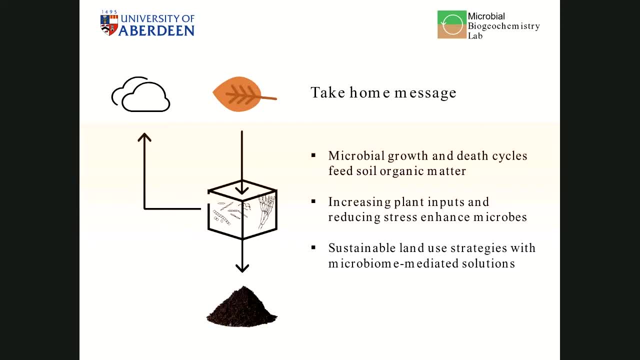 stress in soils will enhance microbes, And that actually, then, is leading to higher soil carbon storage and sequestration. So, in terms, this is not just important as a climate change mitigation factor, but it's also so not just to keep carbon in the ground, but there is also potential to increase. 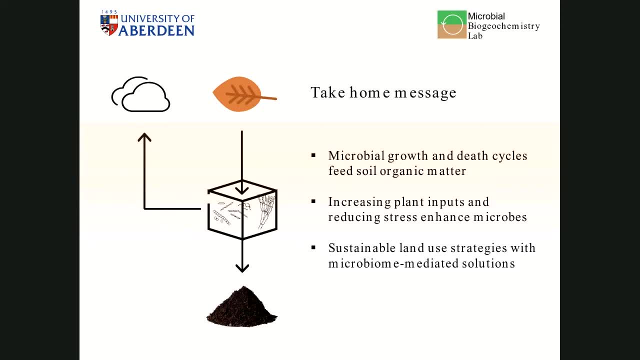 soil carbon because we have large swathes of soils where they are degraded. The carbon content is very low. So there's a large amount of potential there To improve soil carbon in those soils without impacting yields- crop yields- very significantly, because eventually we do need food to feed the growing human population. 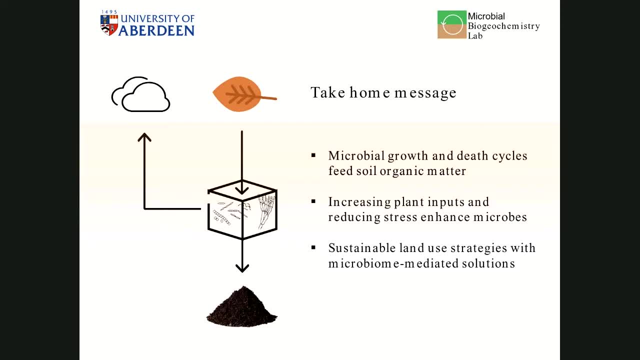 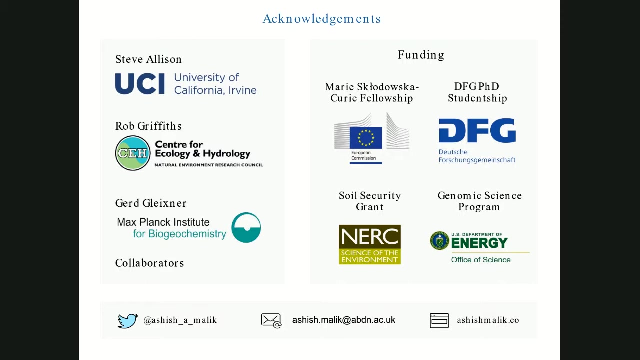 So some of the sustainable land use strategies involve some of these microbiome mediated solutions, because that's allowing us to improve soil health, But also to mitigate climate change With that. I'd like to thank funding agencies that made much of this work possible, primarily. 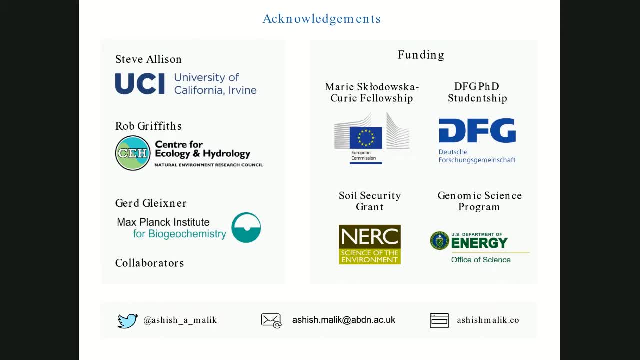 the European Commission for the Marie Curie Fellowship, but also Natural Environment Research Council here in the UK for the grant which supported much of this work, And I'd also like to thank my postdoc advisors in previous affiliations at the University of California Irvine Center for Ecology and Hydrology and the Max Planck for Biogeochemistry. 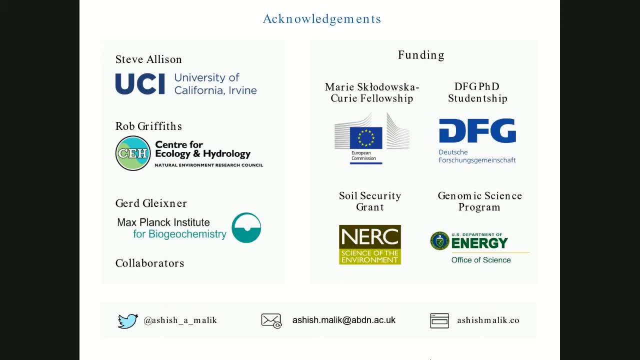 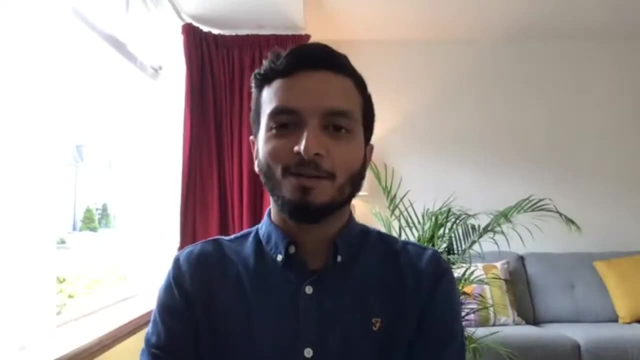 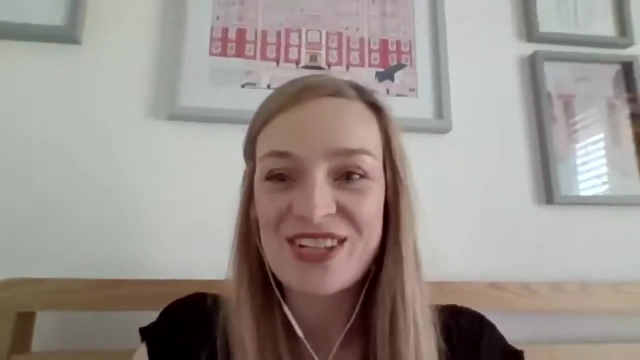 More contact details are here below and I'd like to thank you for listening and joining today. I'm happy to take questions And discuss further Great. I just want to say thank you very much, Ashish, for presenting today and likewise thank 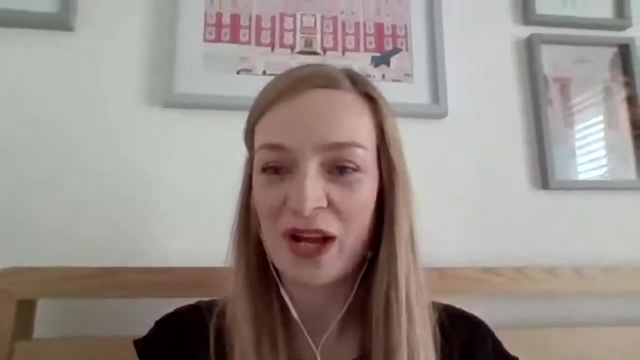 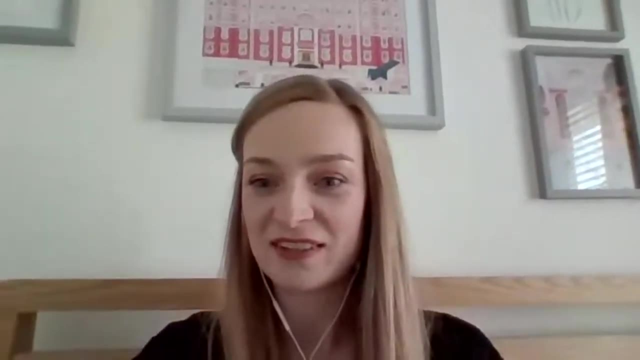 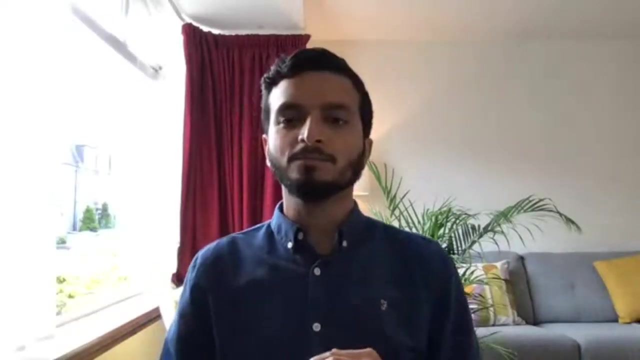 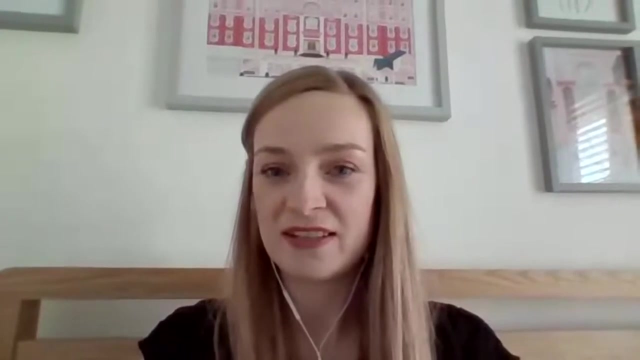 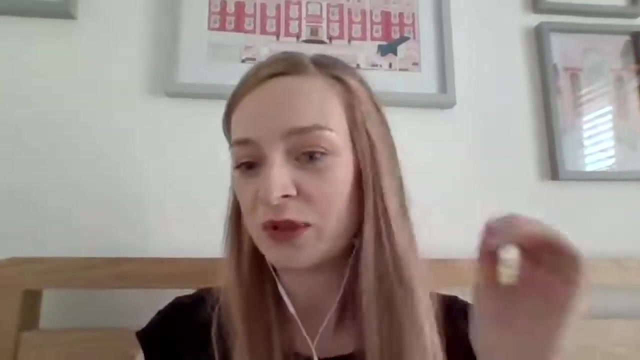 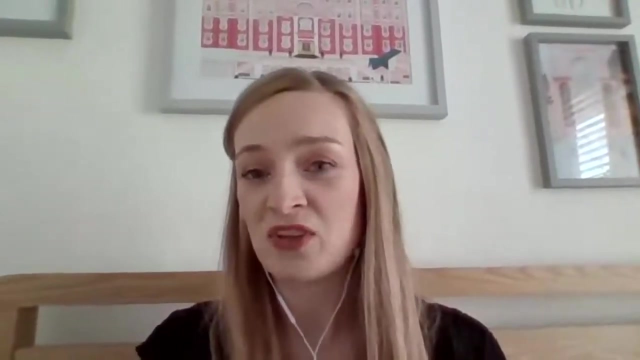 you to everyone for joining. So if you do have any questions, if you're able to type them in the chat box and I'd be happy to read them out. Let us know what you think And I think Next. So 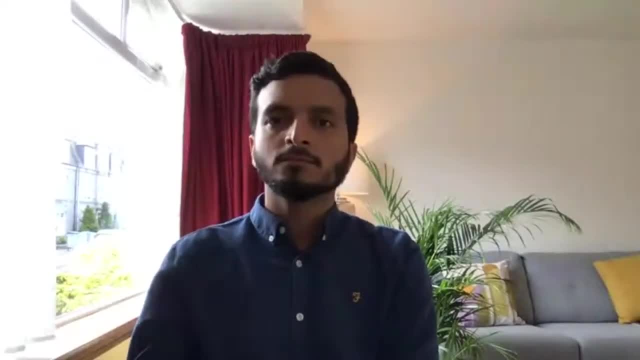 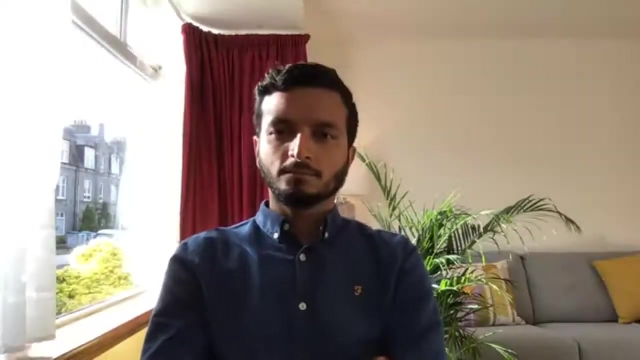 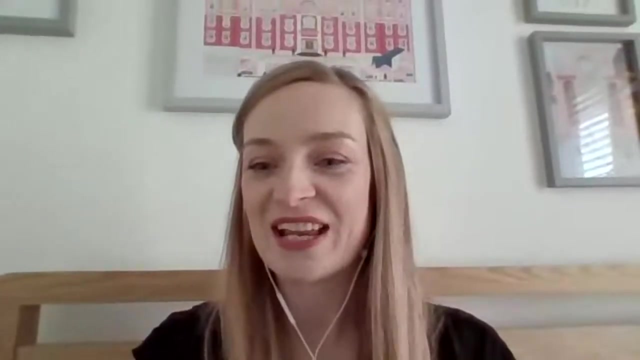 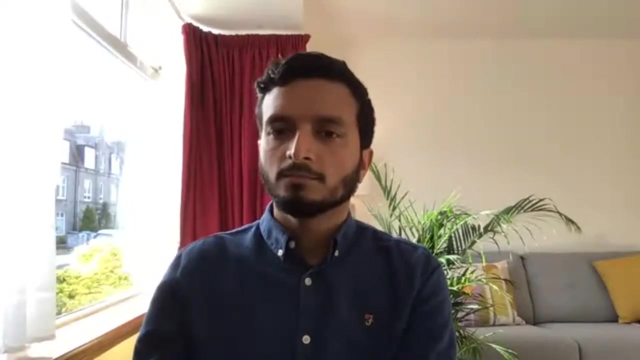 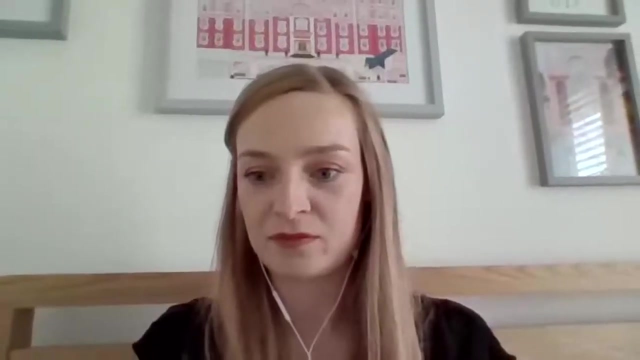 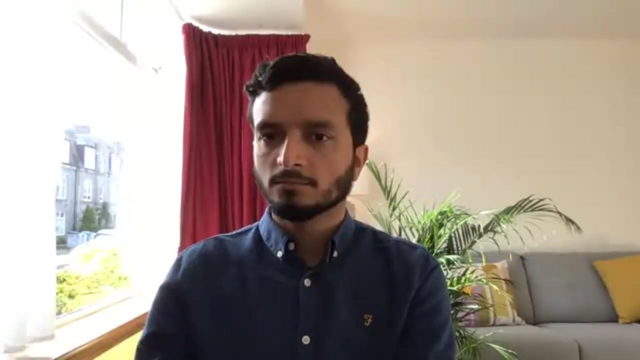 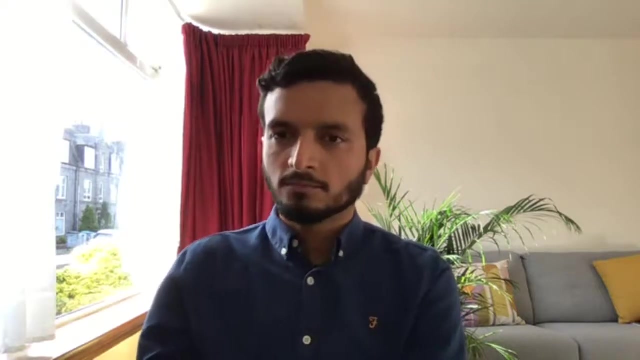 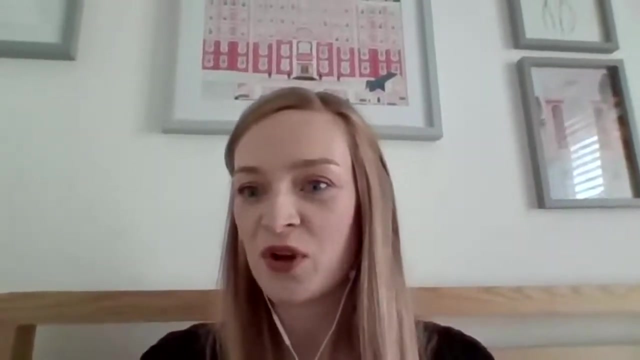 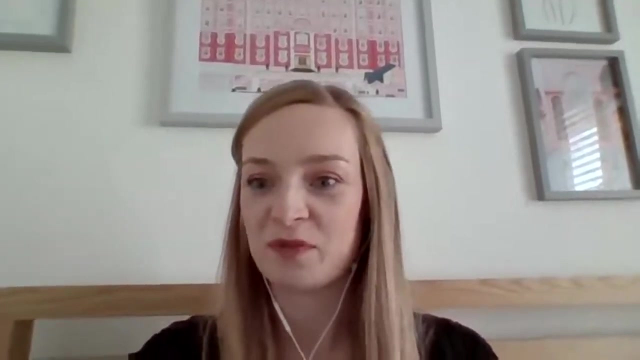 um, oh okay, sorry if you. if you're able to try now and then, that should be work. so we've got a question from richard blackmore asking how great is the potential contribution of increased soil carbon sequestration in helping the uk achieve carbon net zero? 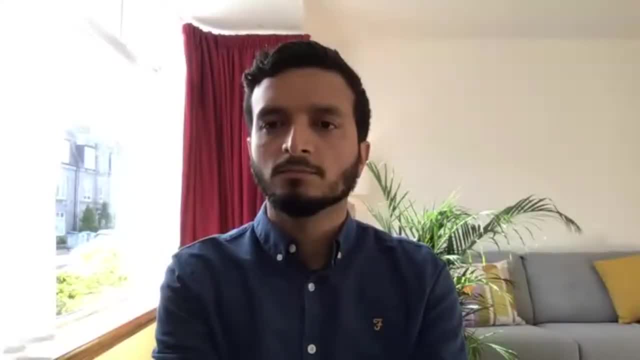 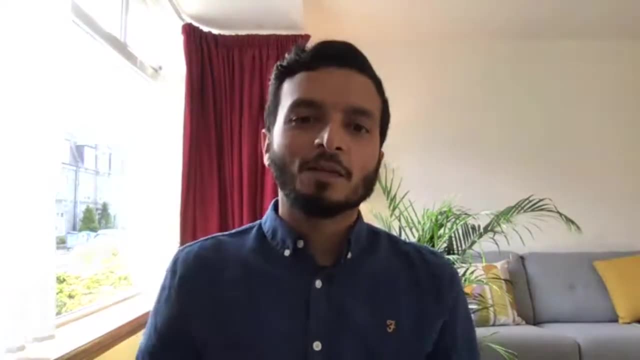 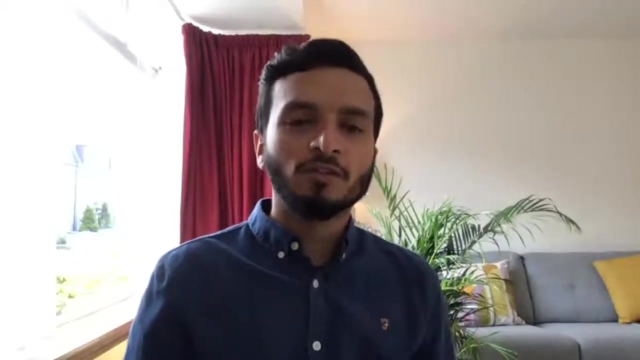 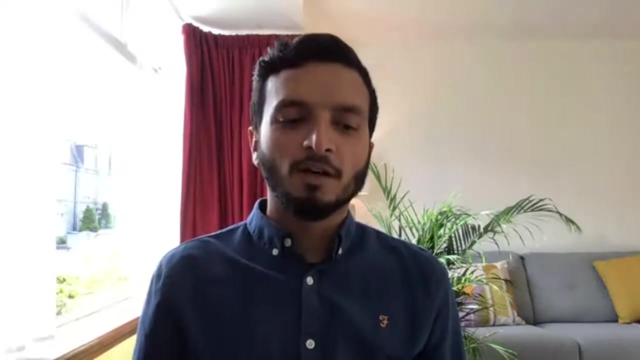 yeah, so, like i mentioned towards the end, um it's uh, there there are a lot of um the swathes of soils in the uk where the the amount of carbon is really low, and this is because of severe degradation through years and decades of very intensive farming. so there is there is an immediate 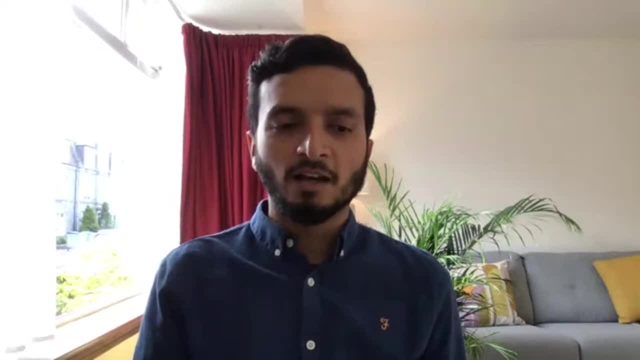 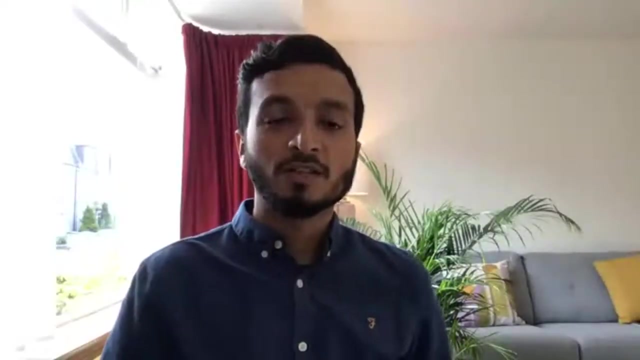 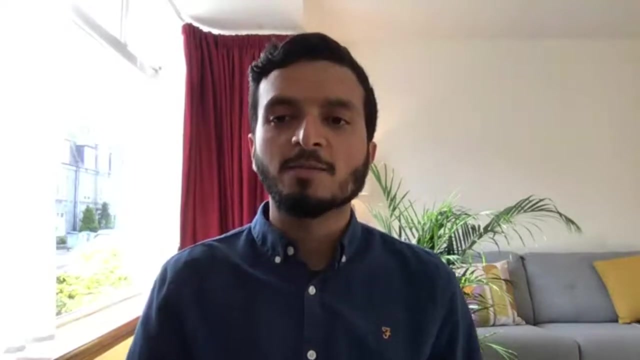 potential there to increase um carbon sequestration without massively impacting crop yields, for example, because this is this is not a massive investment, um because it's so degraded. so in that sense, um that can help us um offset some of the some of the um carbon footprints that are generated generally speaking. 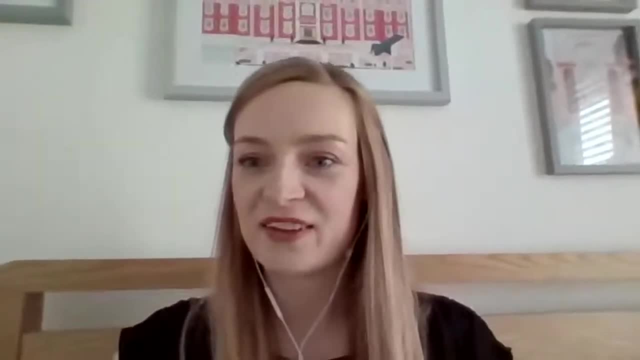 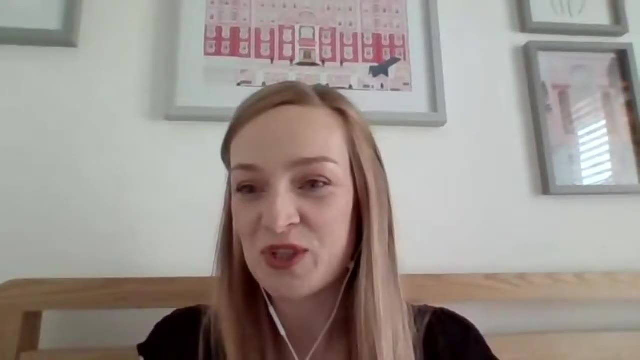 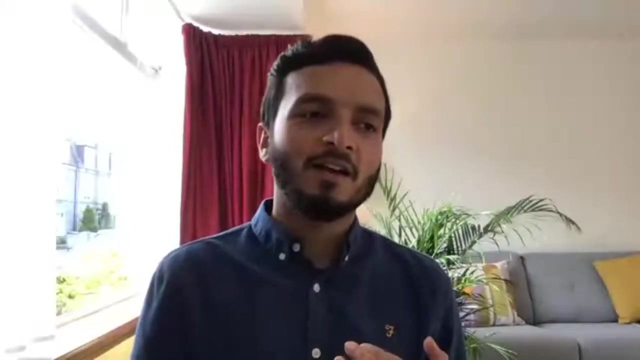 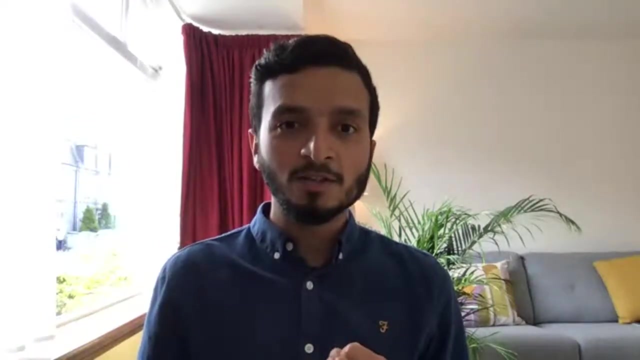 thank you, and there's a question from adam hello, adam, who was presenting earlier. uh, what kind of intervention might a farmer do to improve soil carbon sequestration? biomicrobes said. there are basically two requirements here. one is increasing inputs because we are taking away their food, so various forms of sustainable farming strategies have been tried. 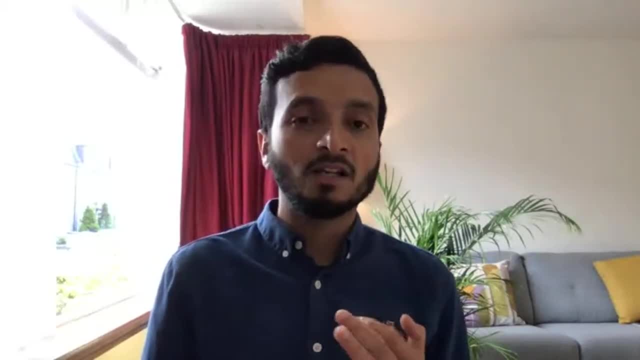 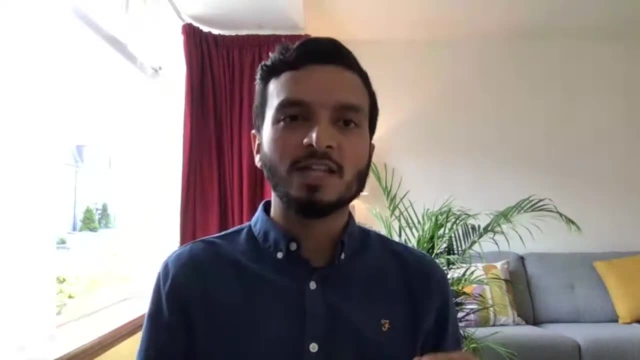 some of them are like involving cover crops. some of them have organic amendments added, so some of these strategies could be useful because they are helping feed the microbes. um, so that's one of the strategies, and the other strategy is reducing the stress, because some of some of the soils 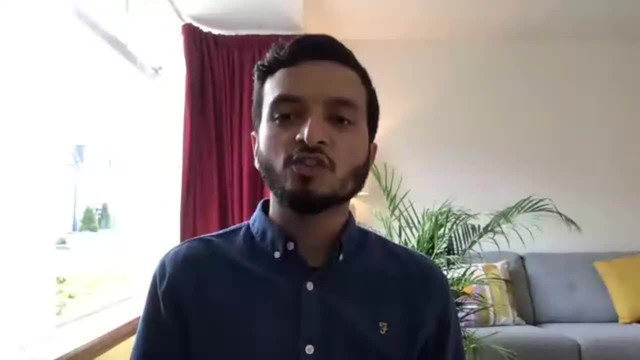 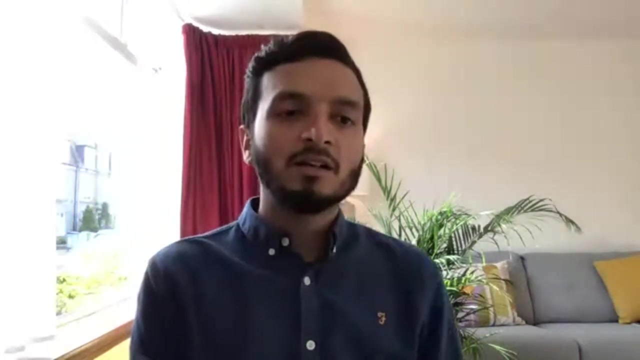 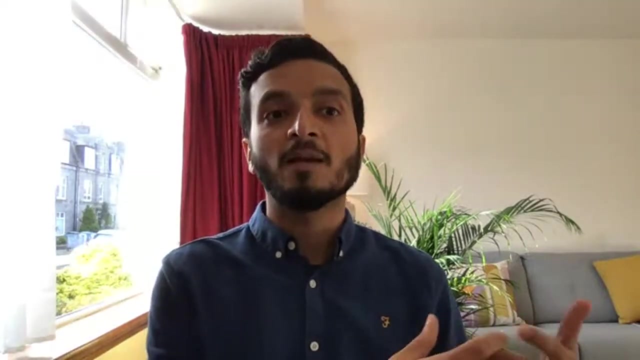 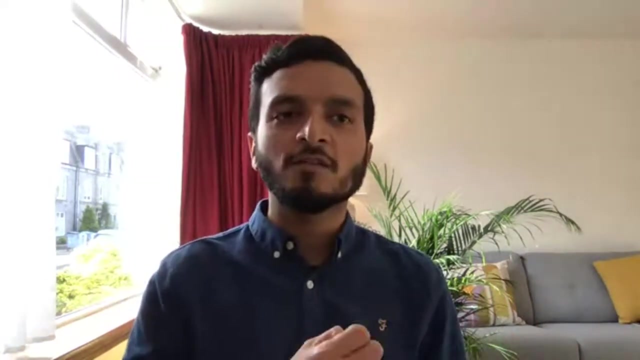 are so degraded that they are very stressful for microorganisms. it's almost like a drought to them in normal conditions, because soils are not being retained there. they are heavily degraded soils. so by building organic matter through microbes, we are also helping the microbes. that again, uh, because that's improving the soil structure and reducing the stress. so it's- it's a reiterative. 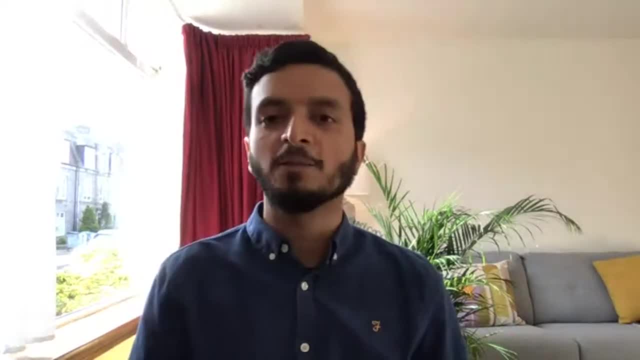 process. it's a feedback that feeds and keeps giving, so by improving organic matter it's also reducing the soil, because then soils can hold the water together, and that means overall it's a very good way to get rid of the burden of the soil. so that's a really good 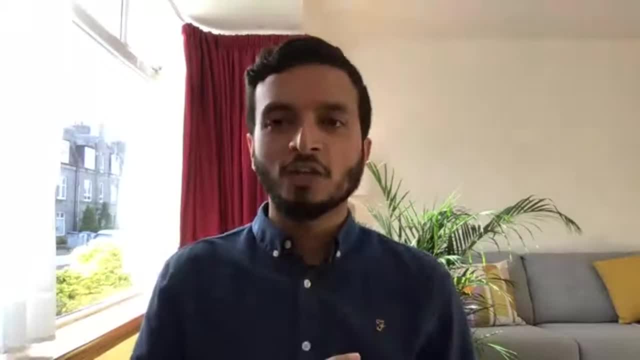 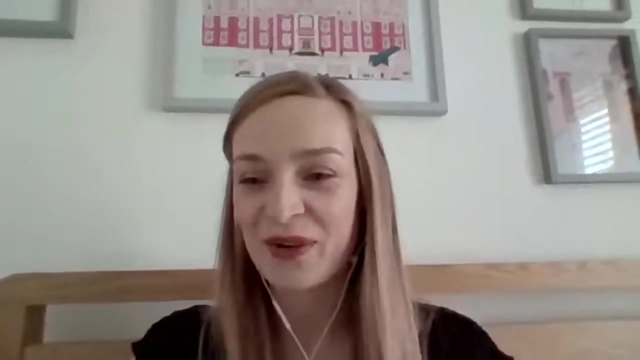 less stressful environment for microbes. So I would say two things, which are both limited food for microbes and reducing stress for microbes, eventually helping them to keep more carbon in the ground. Great, and there is a question from Albert who said: thank you very much for this session. I'm wondering how this research is communicated. 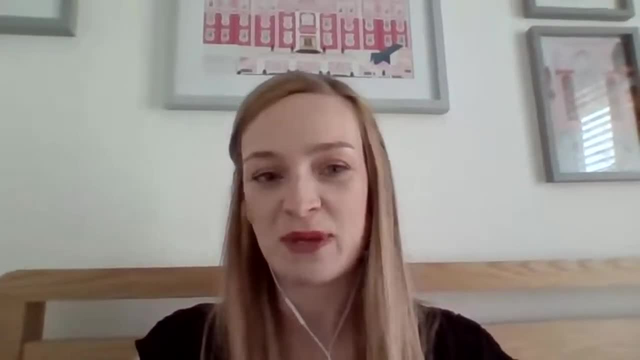 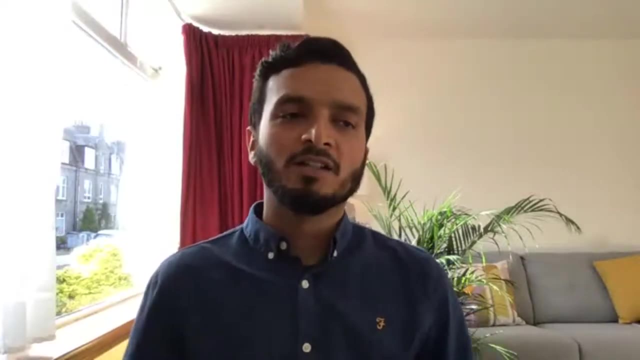 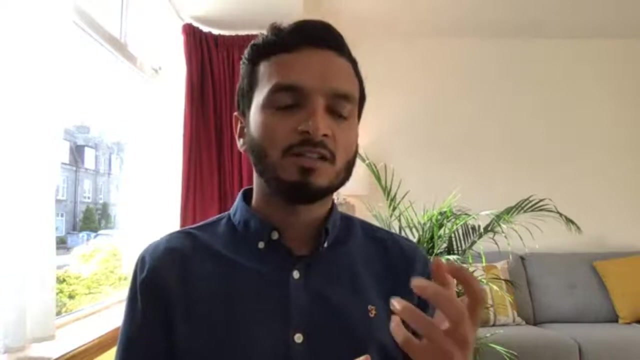 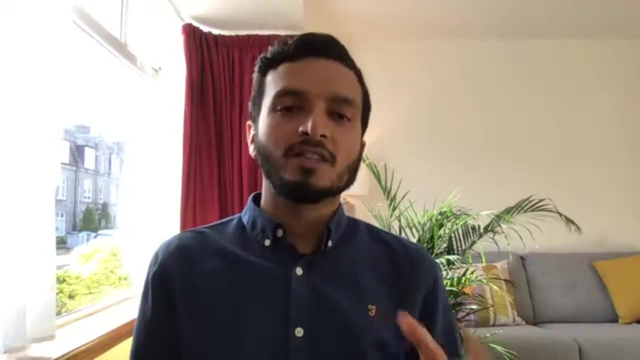 to modern farmers and how successful that has been. Yeah, so some of my work does involve talking to farmers. some of the samples that we've collected are coming from farmers or they are coming from associations with some conservation trusts that are actively engaged in in devising or designing some of these new sustainable land management strategies. 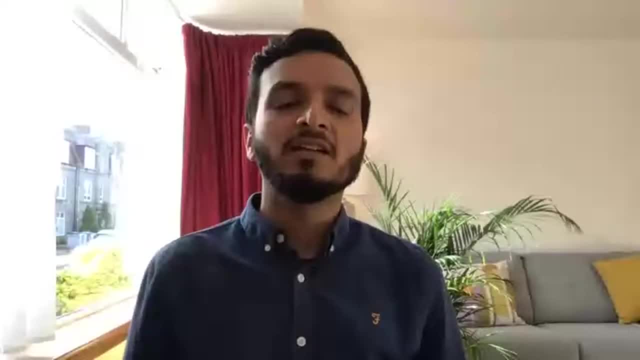 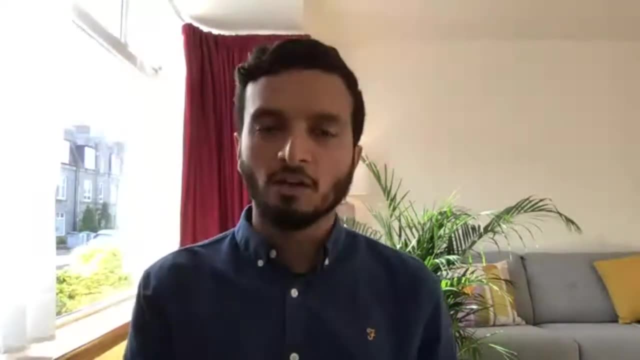 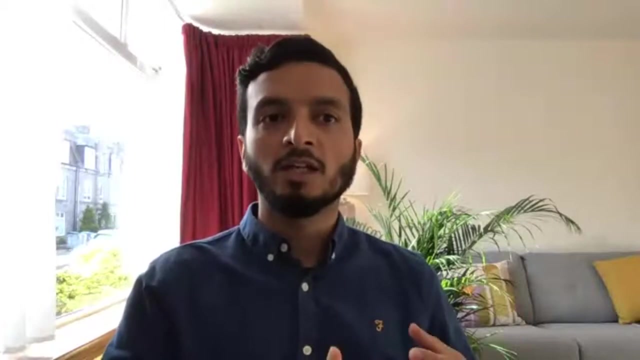 So our work is helping them in understanding if those strategies are successful in ascertaining the success of some of these newer technologies. So this is one way the interaction happens is that they are trying those strategies. we are looking if those are helping the microbes, if those are helping other organisms in the soil. 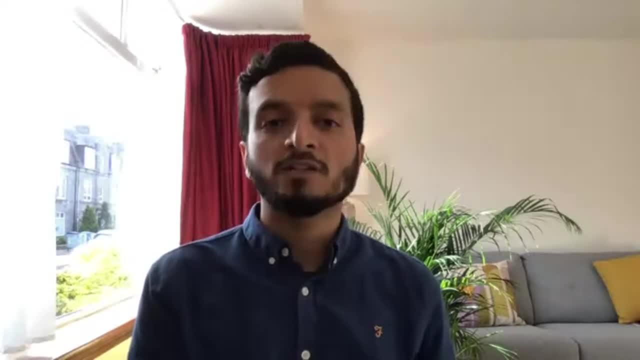 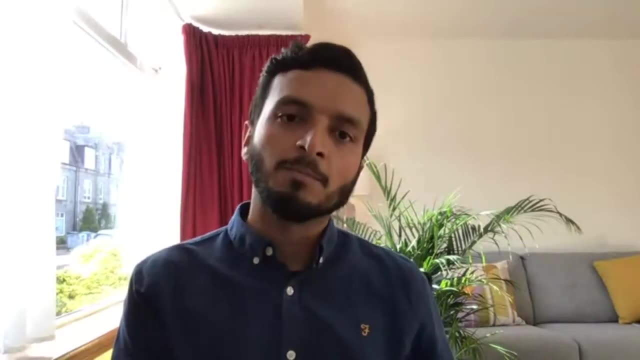 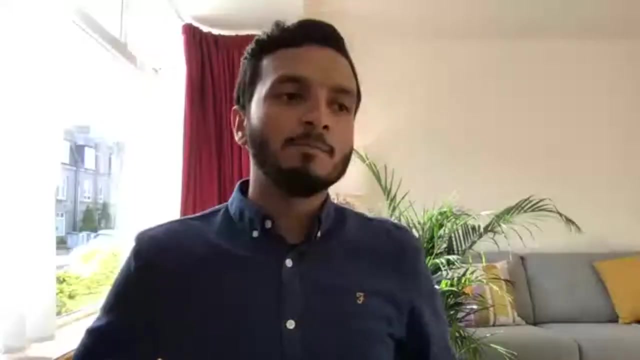 not just microbes, and is it helping us to sequester carbon, is it helping us to improve the nutrient content of the soil, because that then helps the plants as well, And then. so these interactions are important and it's happening, and I'm now writing more. 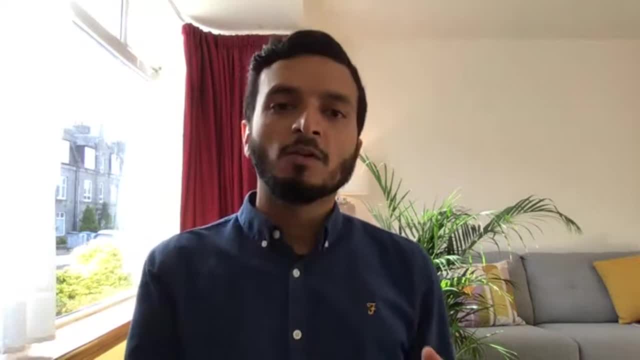 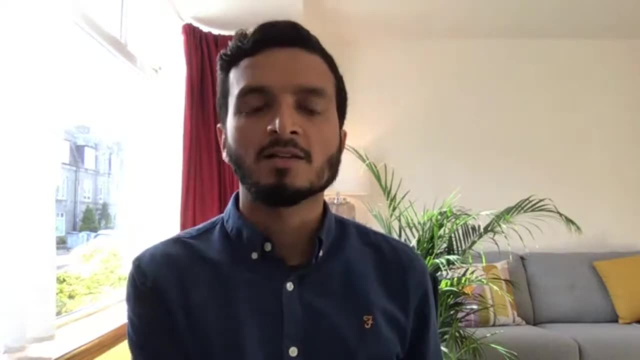 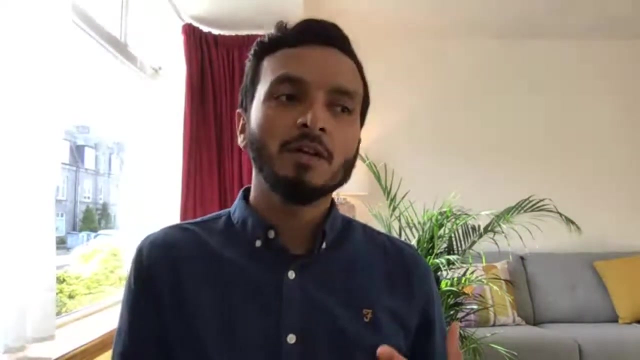 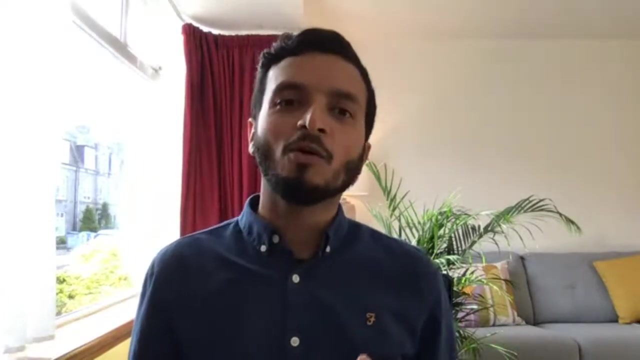 proposals to get funding from the government, and some of these are in active collaboration with the stakeholders, like farmers and policy makers in the agricultural sector. So I think and I'd like to say that some of the farmers are really in tune with some of the latest research and they are actively seeking more information. 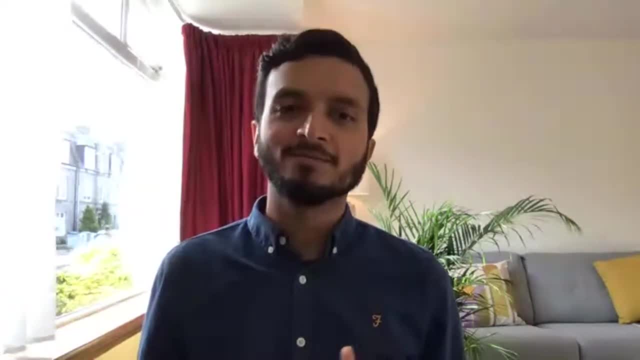 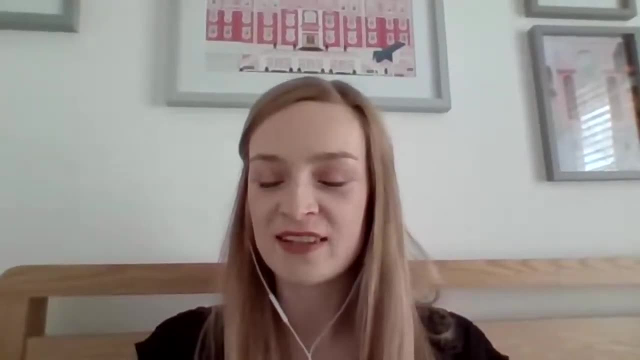 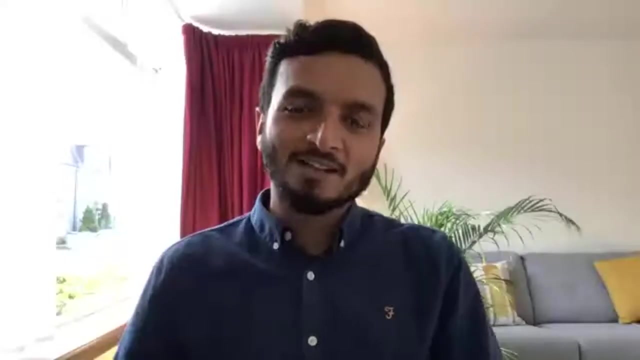 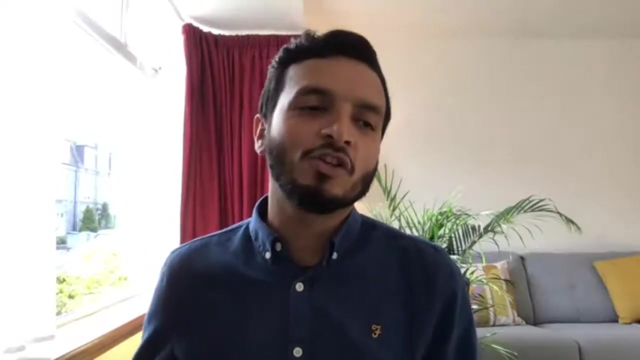 to improve soil health. And our next question is: have you done any soil analysis of the grouse moors of Aberdeenshire? Not yet, but that's one of the projects I'd like to get on with. Actually, there is a PhD student in Aberdeen who's trying to look at some of the controlled burns. 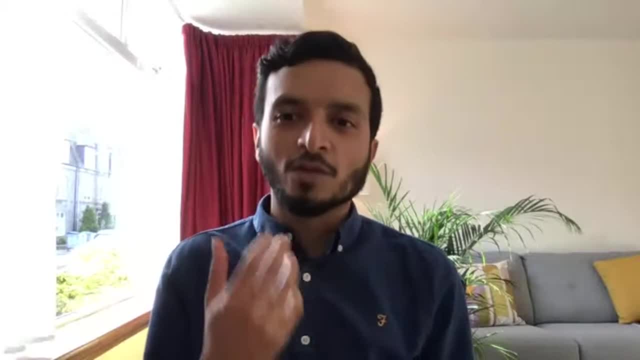 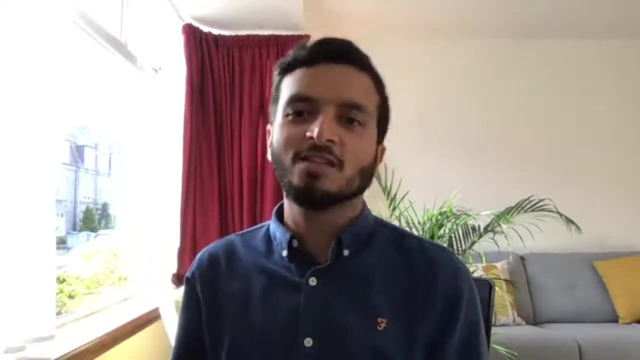 and how they are impacting vegetation, and I was hoping to get on board and look at some of the below ground processes. We will eventually do it. It was cancelled for now. It was cancelled for this year because of COVID-19, but that's one of the projects I'm 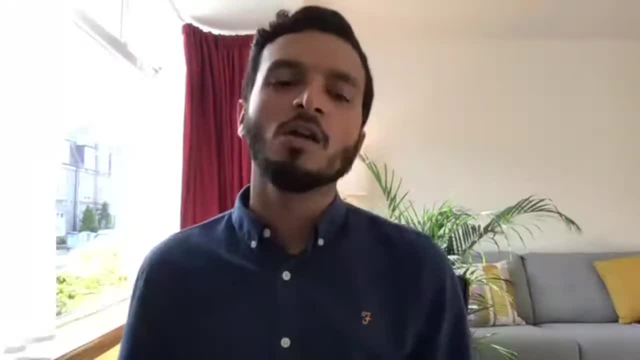 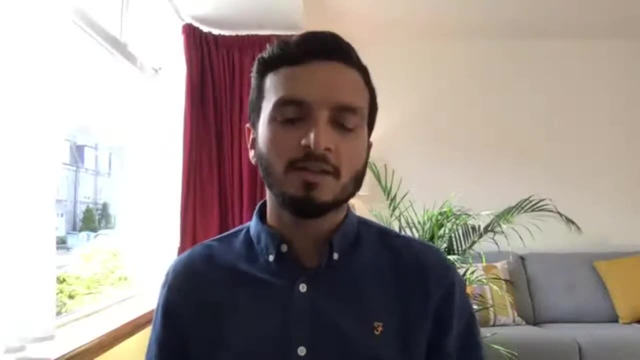 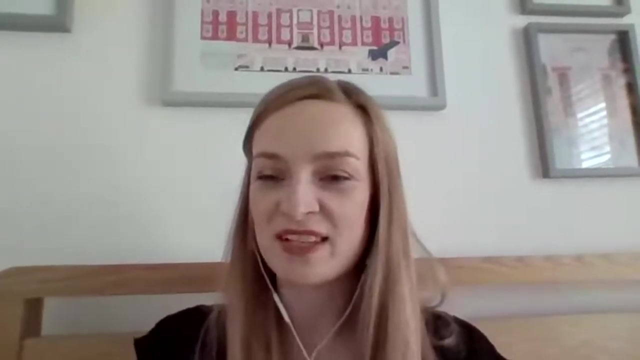 trying to get on board with, Trying to look at how some of these moors can be used to improve carbon sequestration and what is also the impact of some of these burns- controlled burns- on the moors. Our next one is from Tom, who says thank you for your presentation. 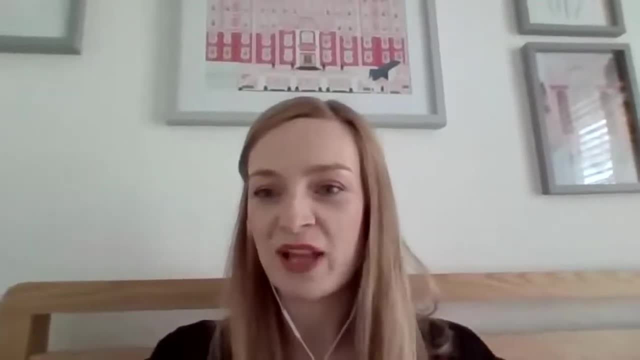 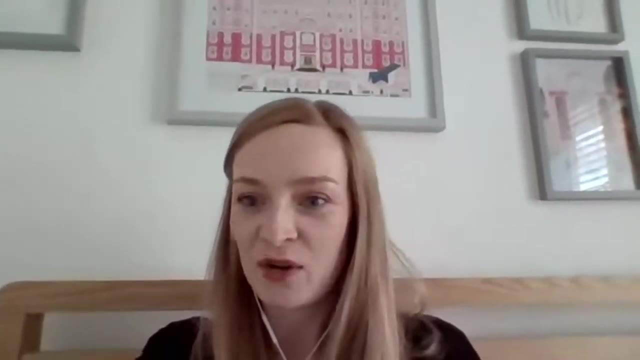 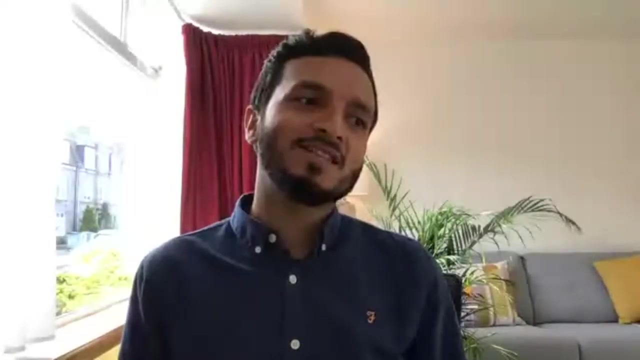 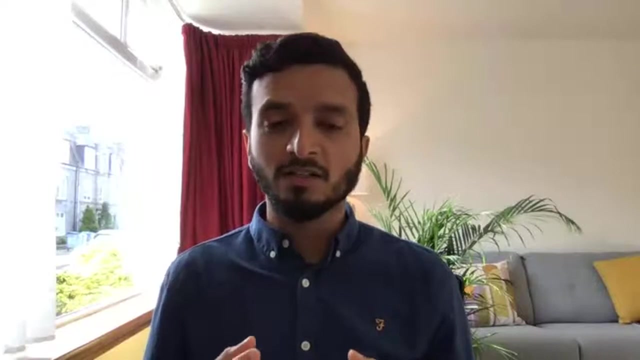 Does the type or quality of plant material that we apply to soil matter for carbon use efficiency and carbon sequestration, or is it just a case of more? I think it's the more the better. Yeah, so yeah, this is a great question. There is a lot of science around the quality of the 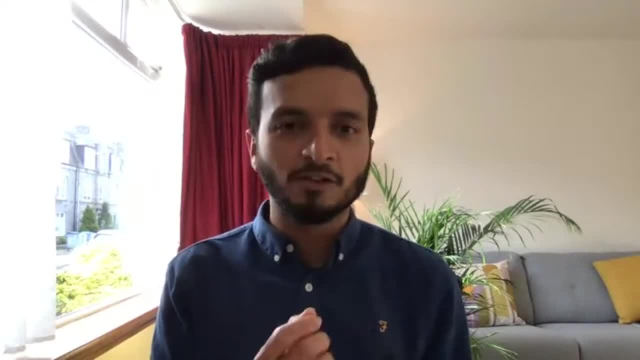 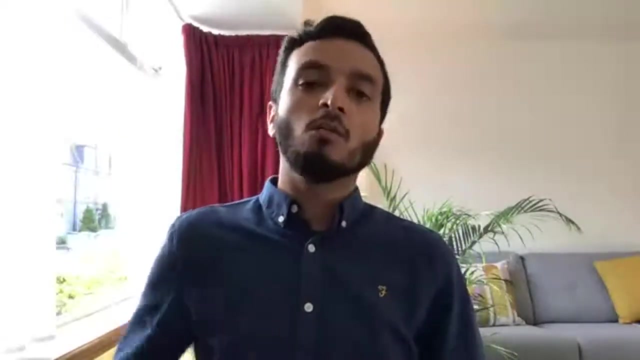 organic matter in terms of the carbon and nitrogen content- So often we use the ratios of CNN- but also in terms of what the what the organic matter is made of. Are there a lot of aromatic compounds or a lot of lipids? or what are the carbohydrates that are present there? This is also important. 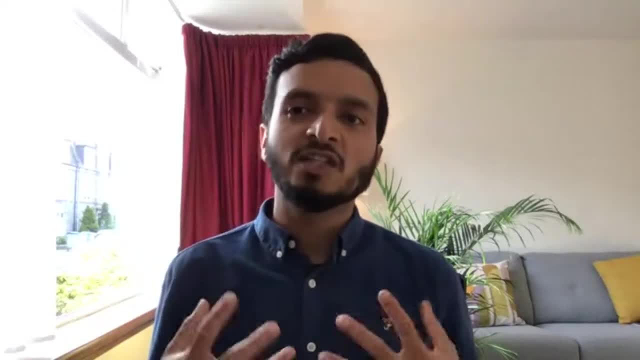 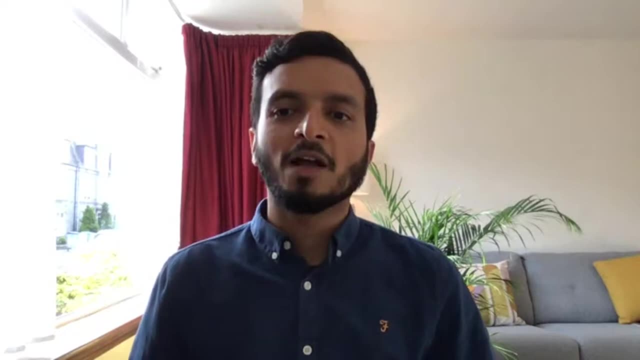 but I think the primary case is that we are just taking away all the organic matter and the microbes are left with no resources, so the so the primary concern would obviously be the be inputs, but obviously there are some inputs that are very, very important, and I think the primary concern would obviously be inputs, but obviously there are some inputs that are very, very important. 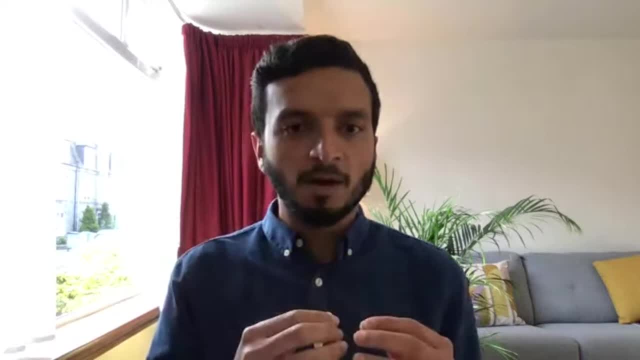 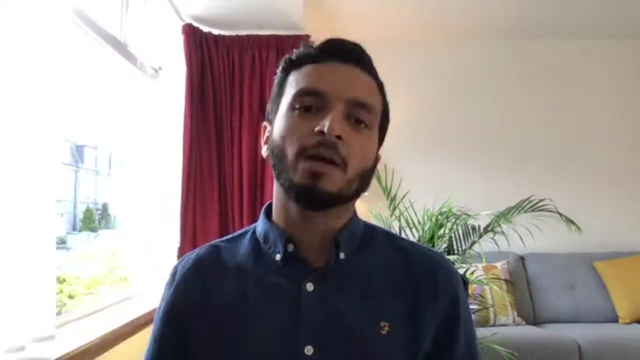 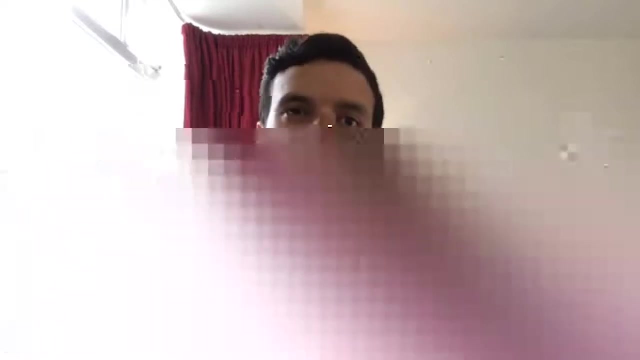 very useful, and if they are less labile in the sense that they're more coming in in in regular periods, then it's better for the microbes. then then some very labile material like say compost that's, that can be very triggering for microbes in certain sense. 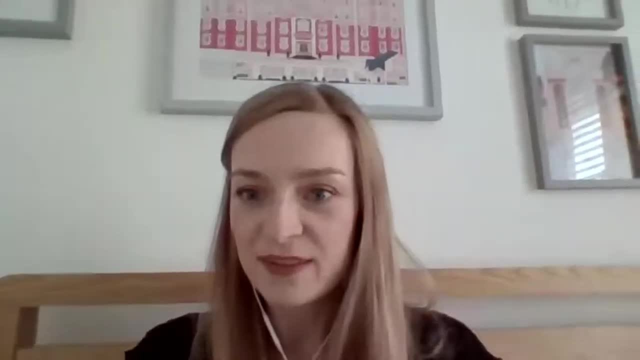 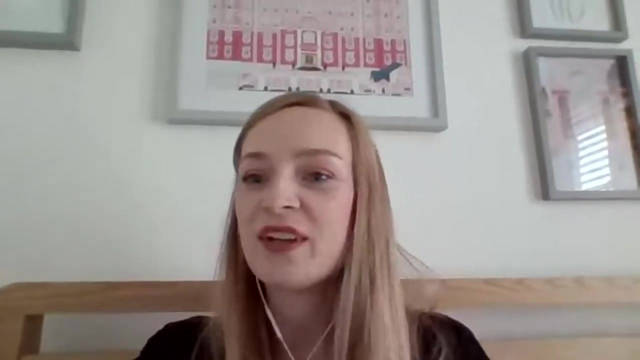 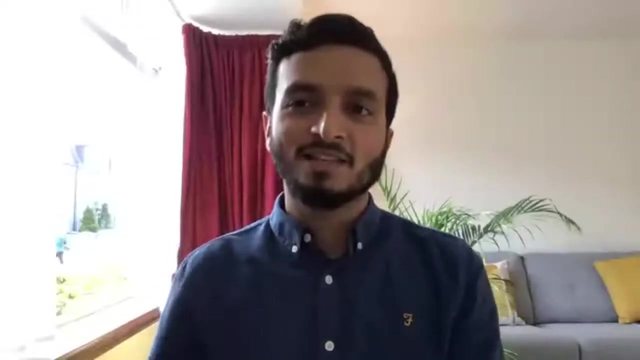 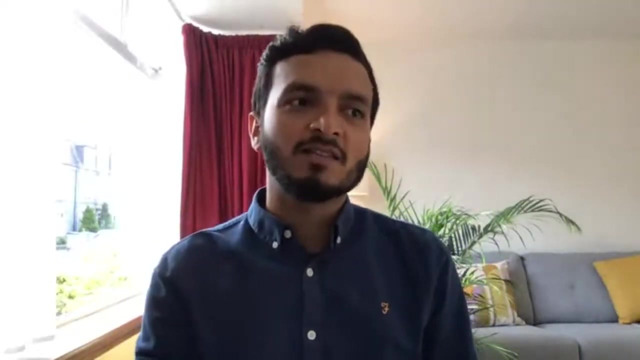 and our next one is from key, saying: nice talk. how do you think the contribution of autotropic microbes and soil to soil organic carbon accumulation? yeah, this is also a fascinating line of research. we don't know much about this, but there are some indicators that they do matter. 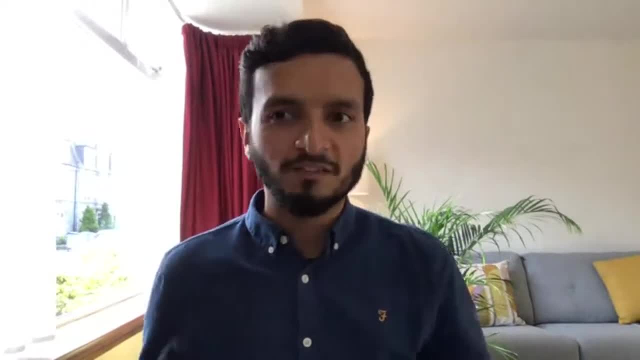 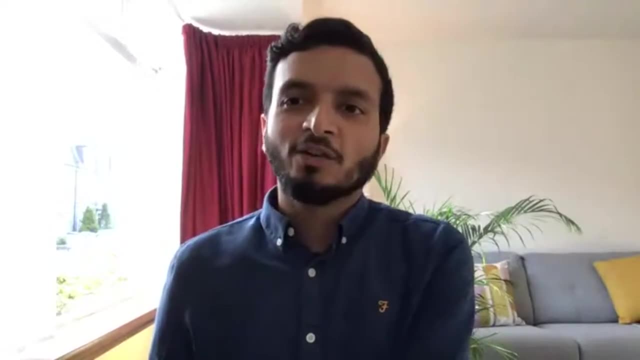 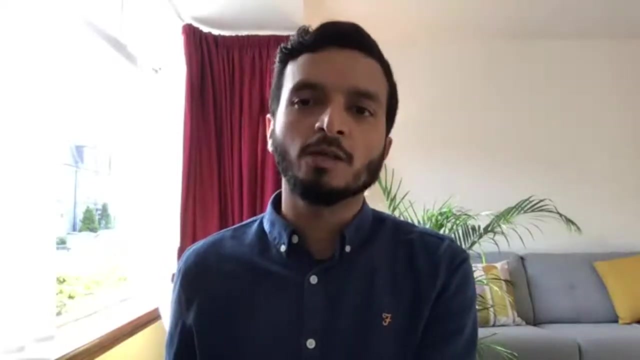 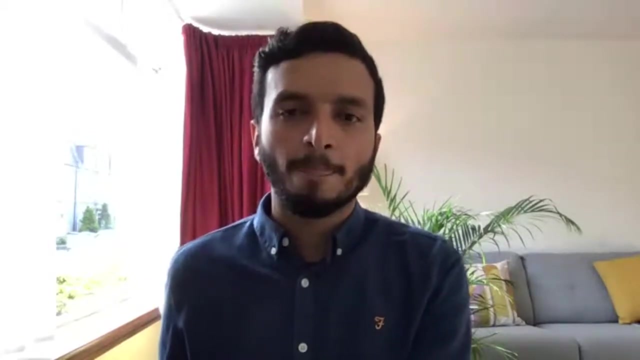 microbes that fix carbon just like plants do. yeah, I. to be honest. I don't know much about the exact contribution, but most of the community in soils is heterotrophic, which is relying on other sources of organic matter, so I'd expect the contribution to be low, if not insignificant. next question is from: 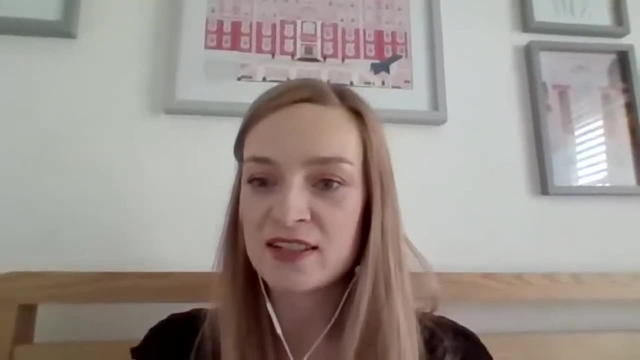 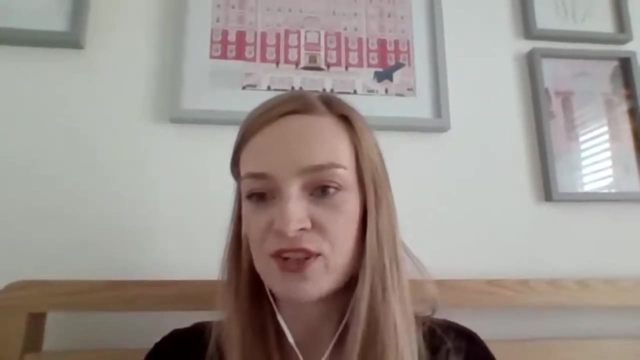 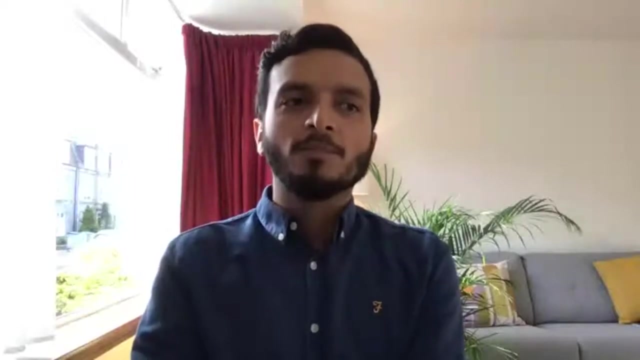 Aftab, who says: has there been any studies conducted to quantify the soil carbon loss due to urban planning? do we know how much of C we lose on average against urban development? yeah, this is also not not a very well developed field of research, but there is. there is some science going on. I'm not very much aware of this, but 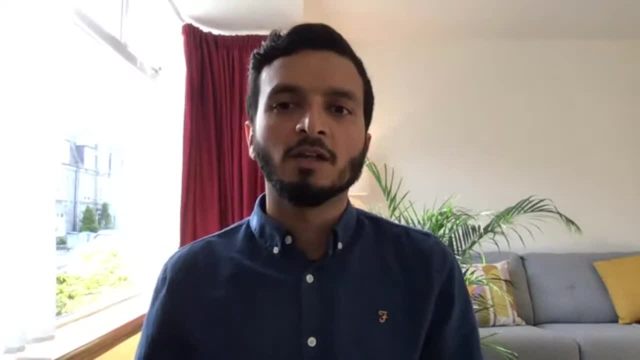 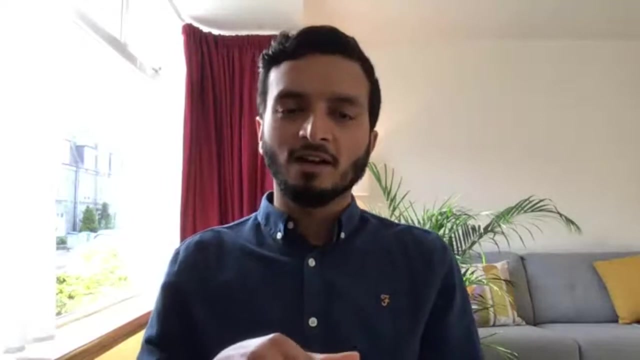 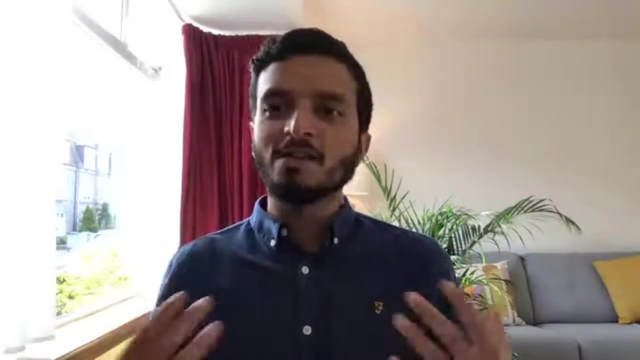 I'm sure this is massively impacting carbon. it may well be that it's posit, it's a, it's a positive contribution in some sense, but I have no idea this is. this is basically almost like shutting off that, that interface between the, the soils and and the atmosphere- right, so this could be. this could be very extreme. 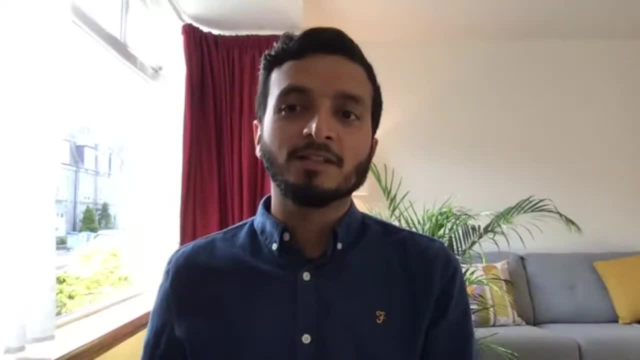 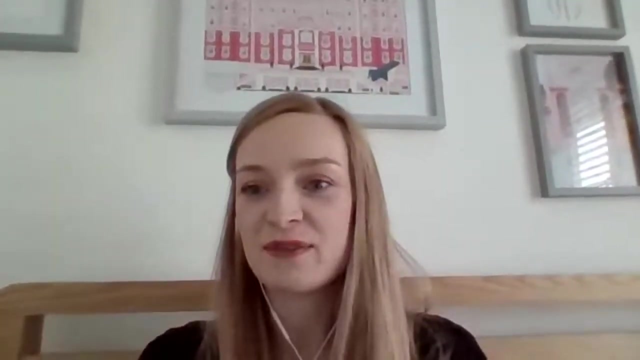 environments in some sense. but yeah, this is this is a very interesting point and they're they're very interesting and I think it should be more research done on that. okay, our next question is: are soils poor in organic matter the best candidates for carbon sequestration practices? 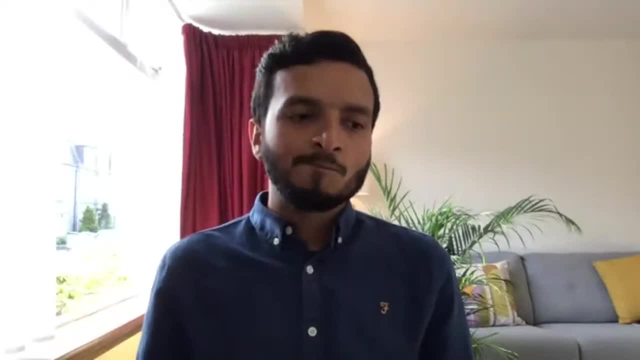 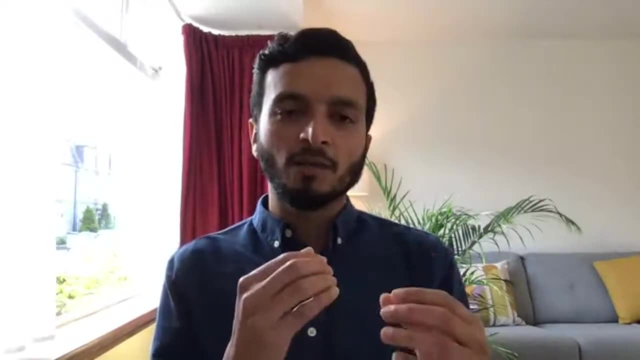 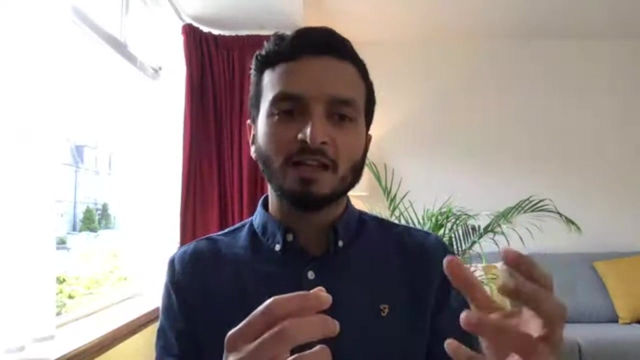 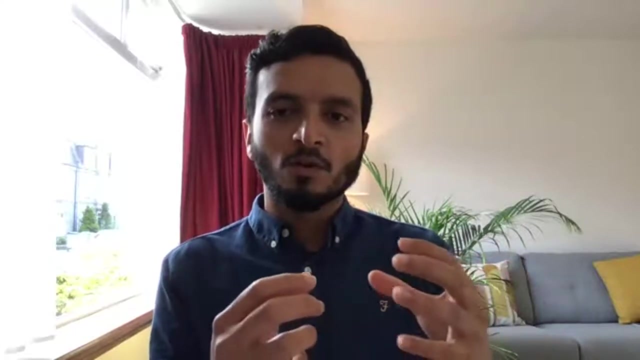 yeah, I say this because because the, the sequestration happens because of aggregation, like organic organo-mineral interaction, so interactions of the organic matter with the minerals. and the organic matter is often some sort of netromass product from microbes. so I say that soils which are degraded are 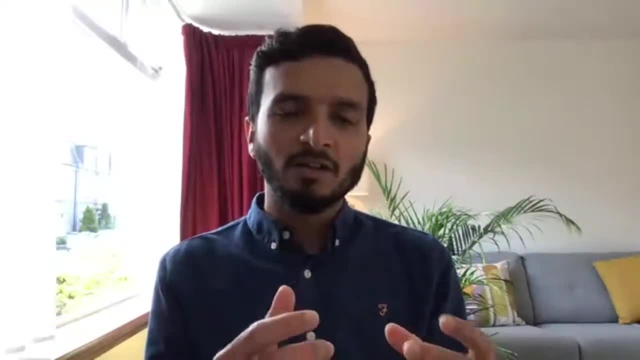 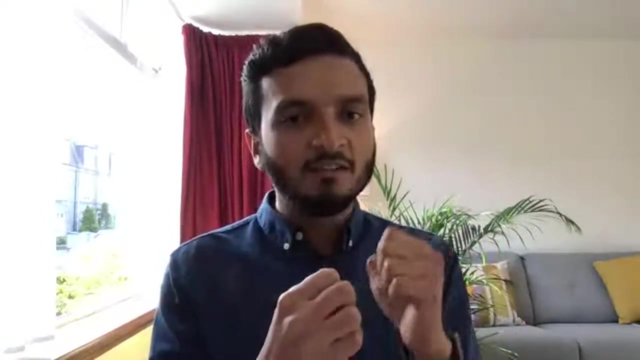 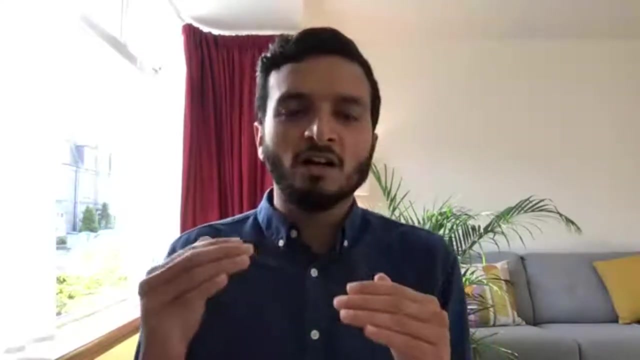 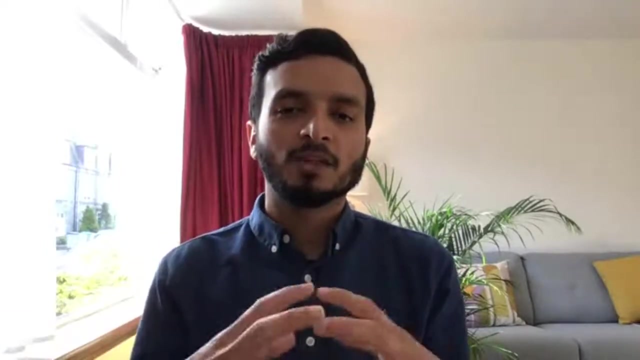 the best candidates because these mineral points are available for sequestration, whereas once you, once you start building organic matter through those interactions, the sites that are available decrease and some soils reach a threshold beyond which they cannot really there are no more sites available for that organic matter. 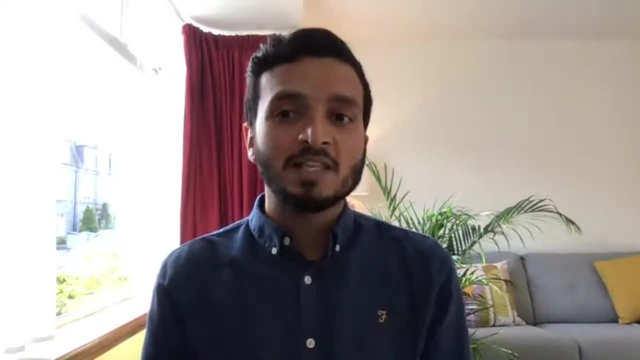 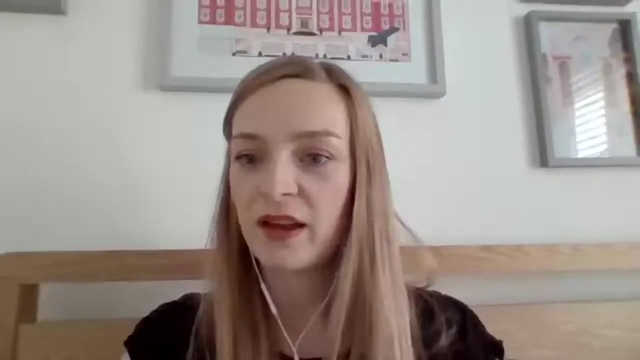 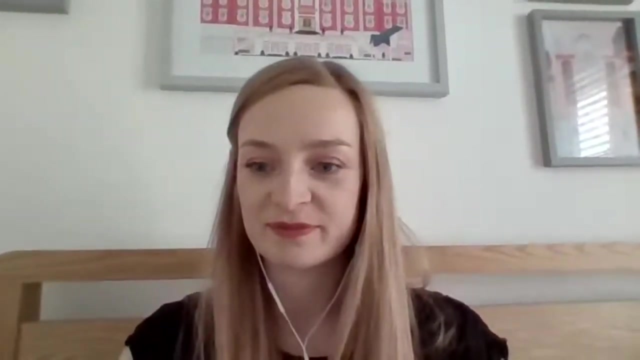 to bind onto minerals. So that's why I say that there is a lot more potential for soils which are severely degraded, because microbes, if they are given a chance to grow and survive and thrive, they can easily build organic matter. Our next question is from Bob, asking how destructive is ploughing to organic matter reduction? 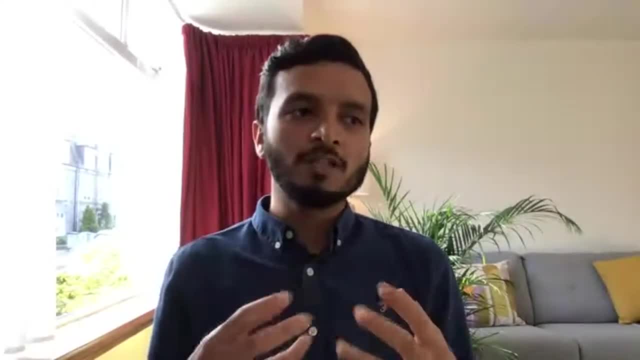 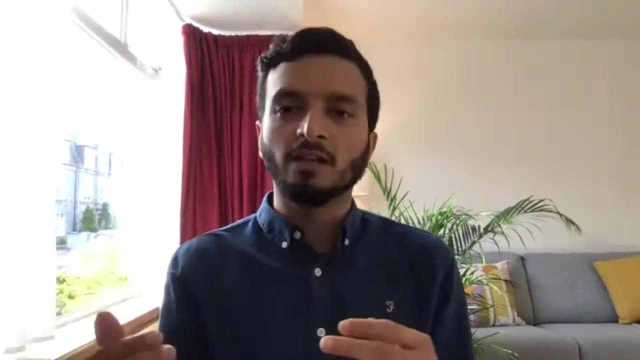 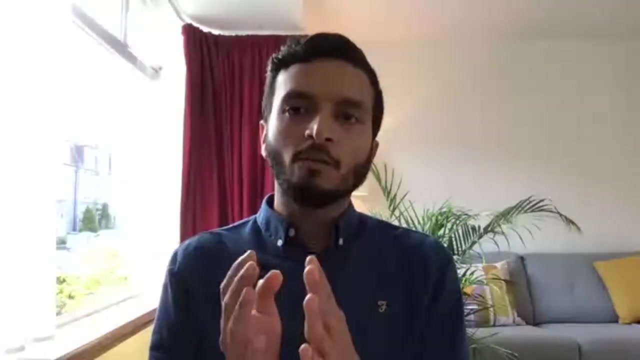 Very much so. And a lot of these, These, A lot of the mechanisms for loss of carbon are physical and chemical and that has very little to do with microbial processes. So when we go from a nice rich organic- you know organic- rich soils to a degraded 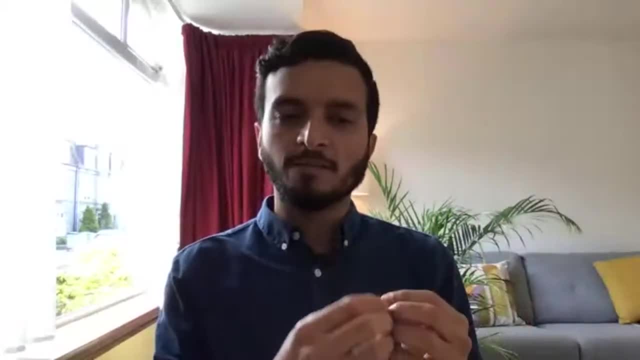 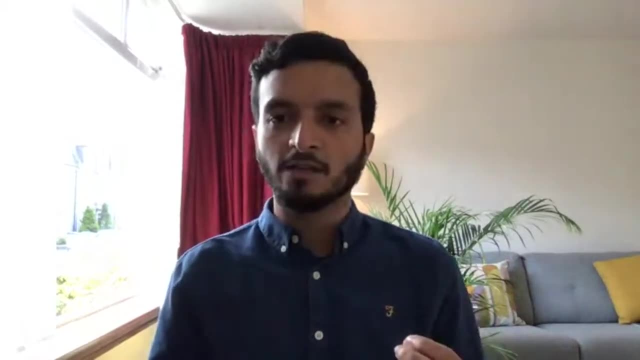 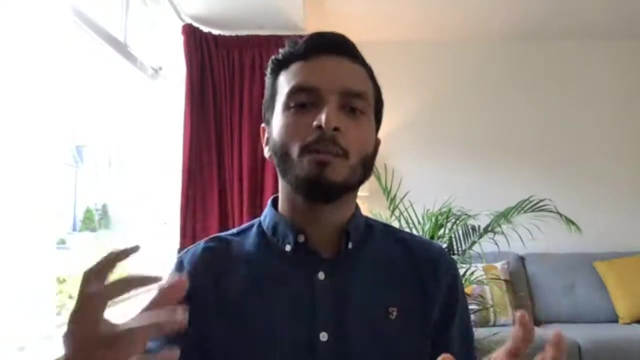 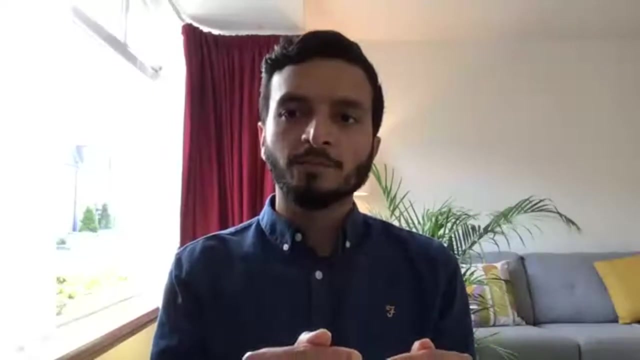 soil. it's mostly because of tillage and all these intensive practices which expose the organic matter to degradation, be it microbial, biological or chemical or physical. But the the process in the other direction is largely microbial. So going from degraded back to rich soils is is it's largely microbial. and so I'm saying 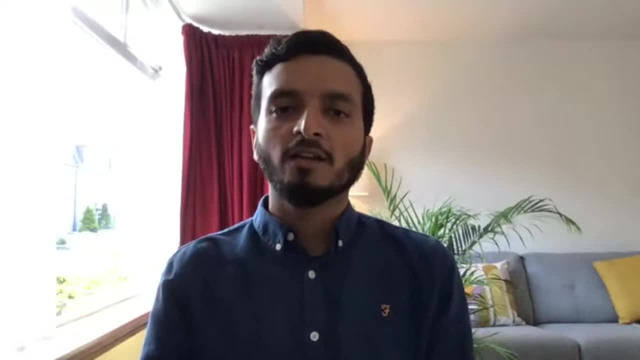 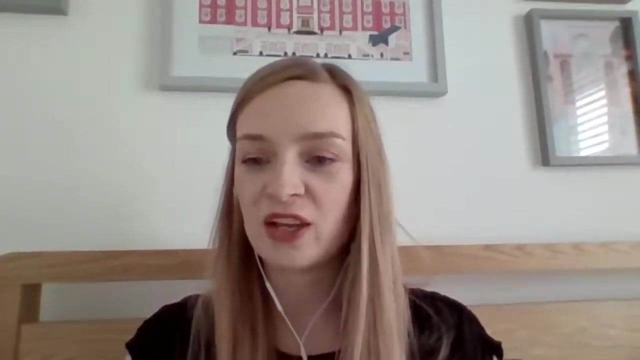 that there is a significant potential there to mitigation. But if you want to prevent loss, it's some of these strategies that have to be minimized. But if you want to build organic matter, Then it's the biology that rules. And our next question comes from Mary, and can you please explain what you mean by increasing? 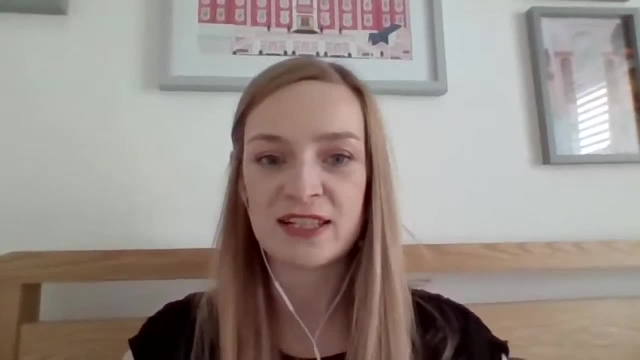 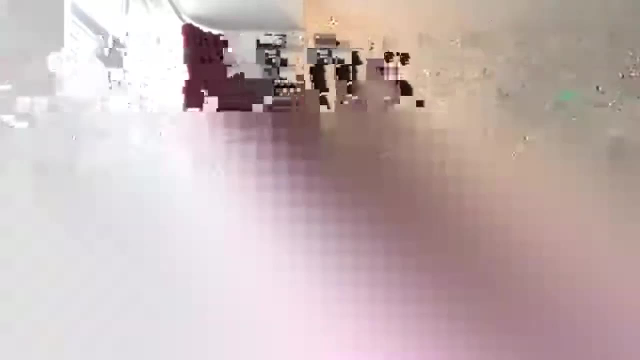 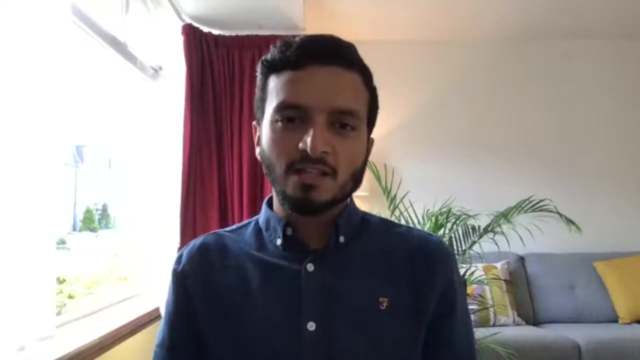 plant inputs. I assume you don't mean standard fertilizers. No, what I mean is generally how how plant soil interactions happen. is plants give my give out root exudates into the soil, And it's often for their own benefit. They form interactions with arbuscular mycorrhizal fungi. 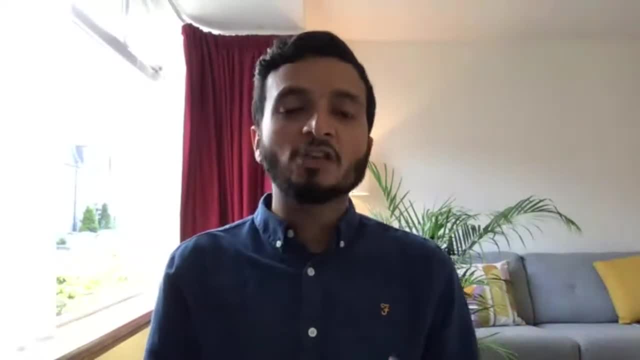 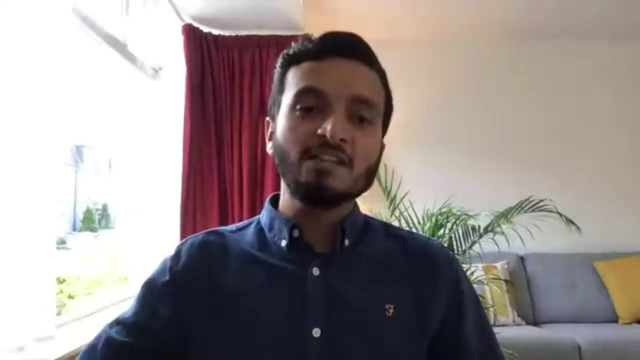 They have a lot of microbes in the rhizosphere which are actually aiding in their growth, helping them fight pathogens, And so these root exudates are important, But also when plants give they because of leaf fall or just even the root litter, when 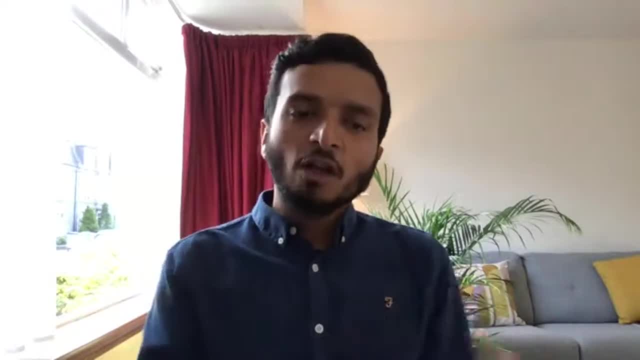 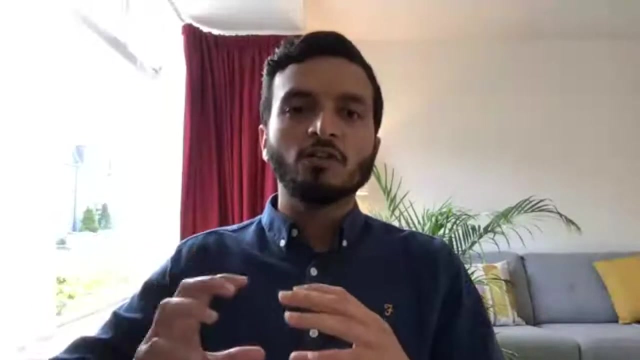 plants die or that they senesce All that That material is available for microbes. But in an agricultural setting, what we are doing, we are maximizing crop yield, We are maximizing food production. So we are not really thinking about the whole system which is feeding the plants as well. 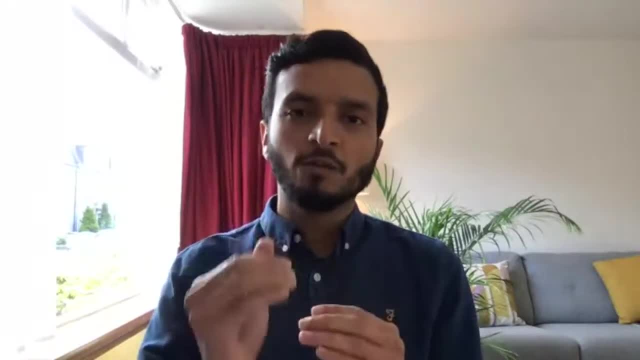 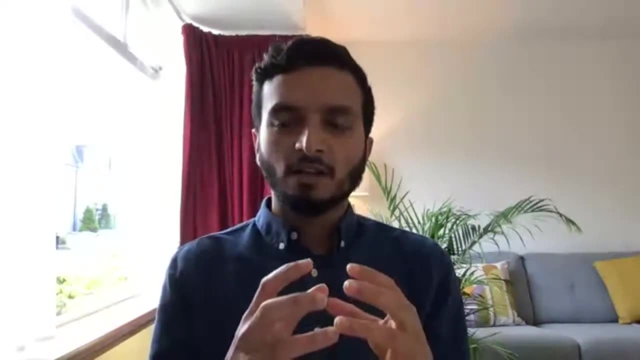 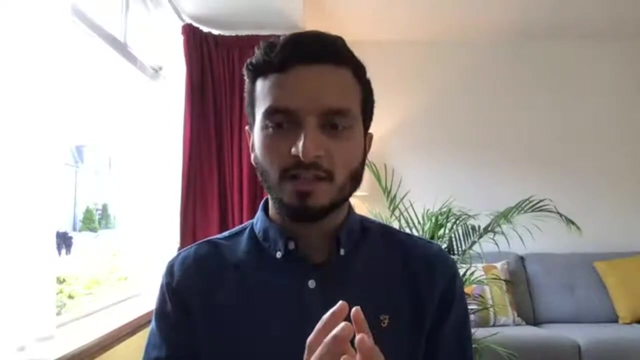 We are only looking at how best to get the foods, how best to get the grains or the seeds. So that's why I'm saying that We need to return to some of those, some of those natural equilibrium processes, and that's why plant matter inputs are important, rather than taking away everything, some of it could. 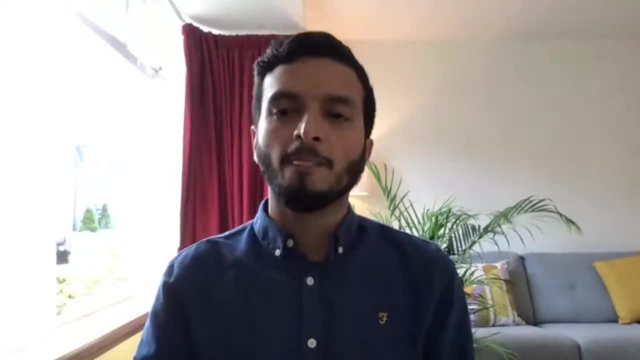 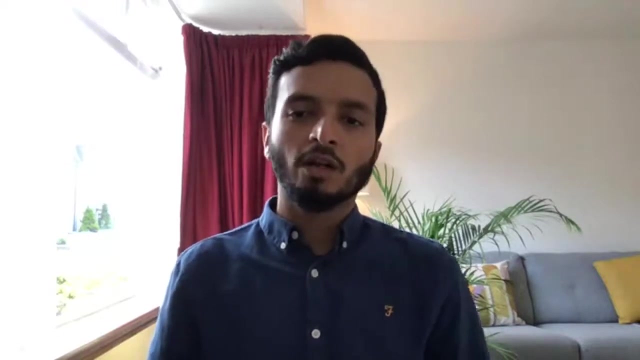 be left. Obviously, it's a big investment, but but if it helps to keep soil health, that is one of the strategies to to employ. Yeah, it's not fertilizers, because that's just bypassing the whole system. Yeah, It's just bypassing the whole process of acquiring nutrients for plants. 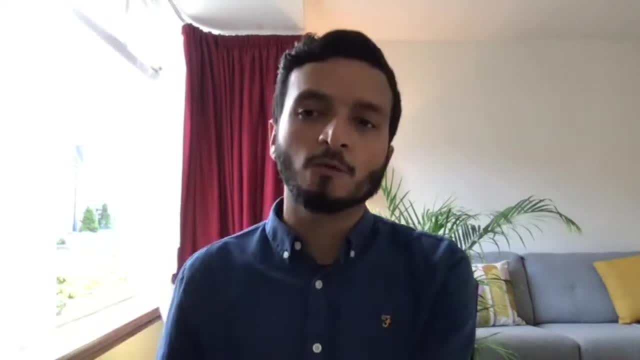 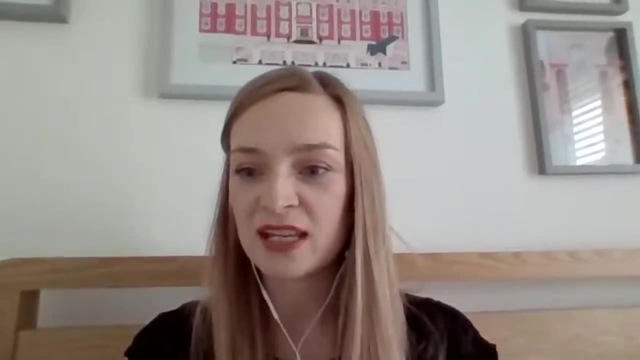 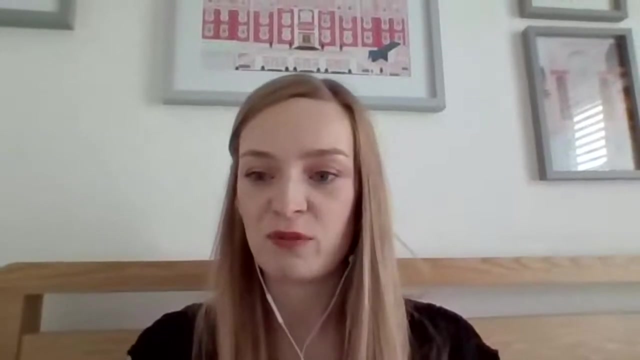 And it's not not helping in the in the long run to improve soil health. All right. Next question is from Bill. With regard to maintained landscape areas, would leaving leaf fall slash grass cuttings in situ improve microbial action and carbon sequestration? 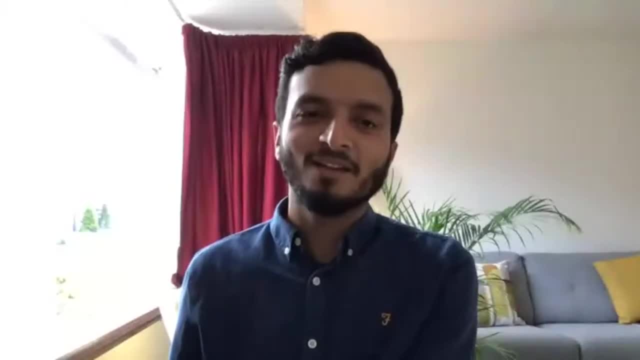 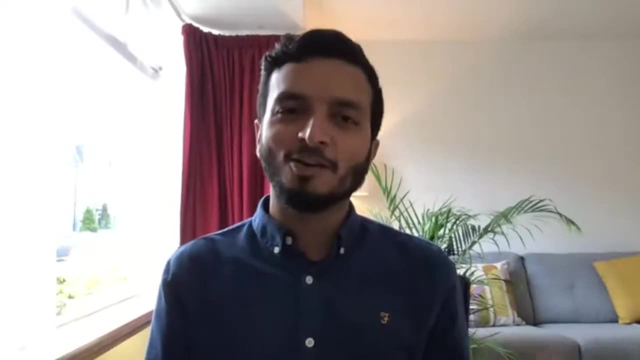 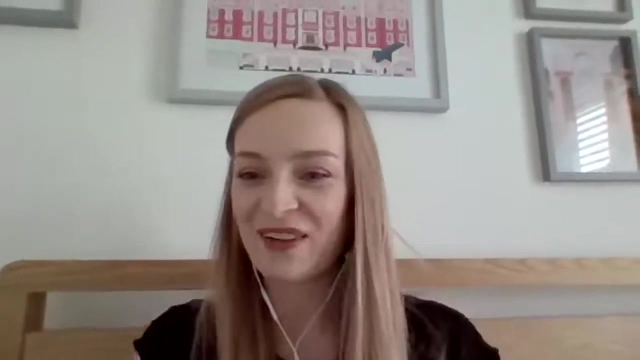 Absolutely yes. Yeah, That's why I leave some of my grass when it's cut back there, so that the microbes have food as well. And do we have? yes, we've got another question from Aftab. and do the green space management? 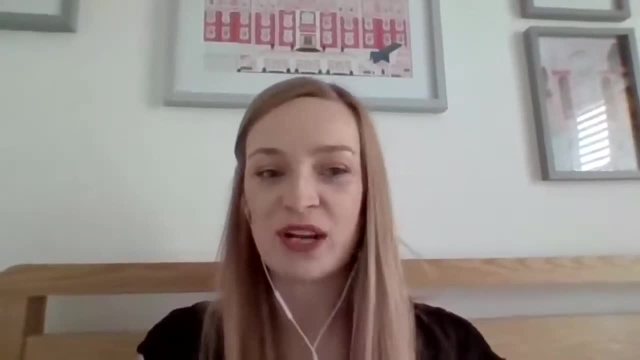 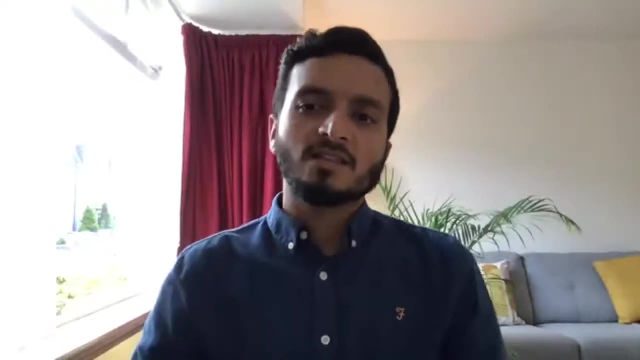 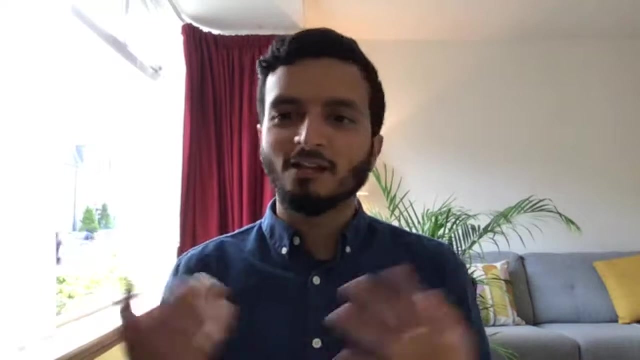 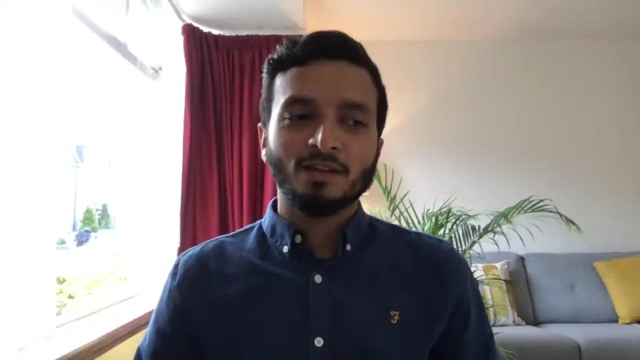 practices affect soil carbon, for example, grass, cutting grass, Yes. So, like I just mentioned a lot of these, yeah, a lot of landscaping uses a lot of water, And we are, yeah, it's, it's a disturbed environment, so to speak. 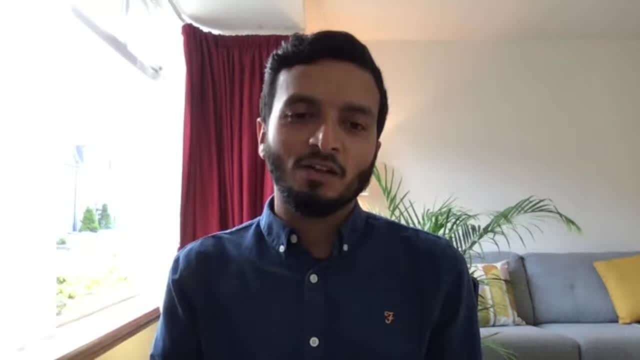 And, yes, cutting grass. We are taking all the organic matter away, then, And it's it's disturbing the balance of those plant soil interactions that I that I just talked about. So, to improve organic matter in the lawns, in the green spaces, we will have to return. 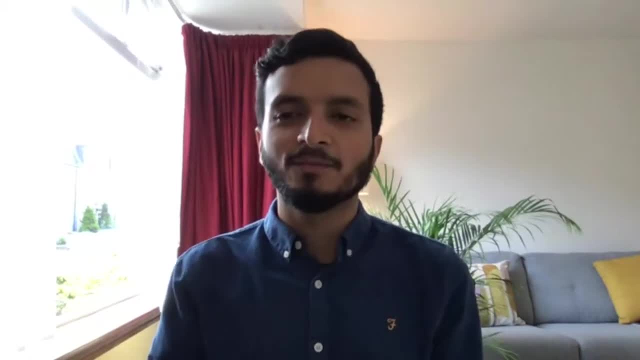 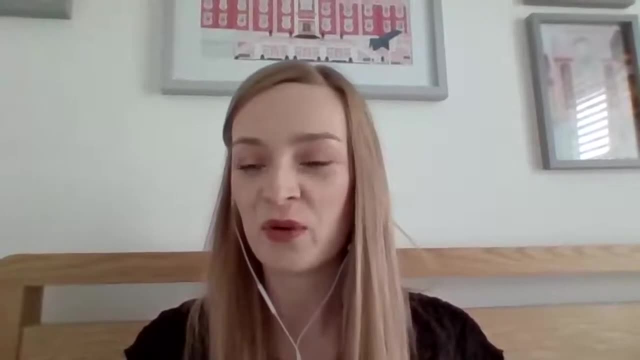 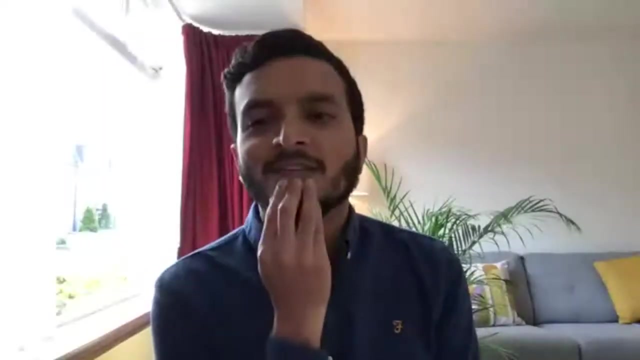 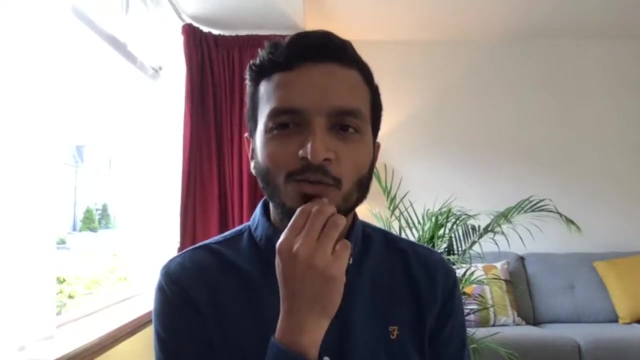 some of that organic matter back to the soil And we just had a few more questions. So why do you tropical soils with low organic matter still produce good crops? Oh, that's an interesting question. I would argue, maybe, that the mineral nutrition is better there, but I'm not very sure. 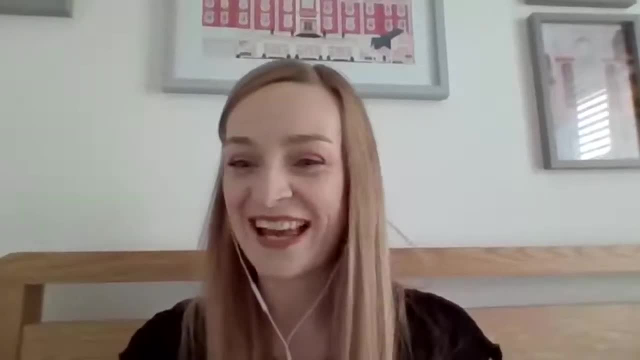 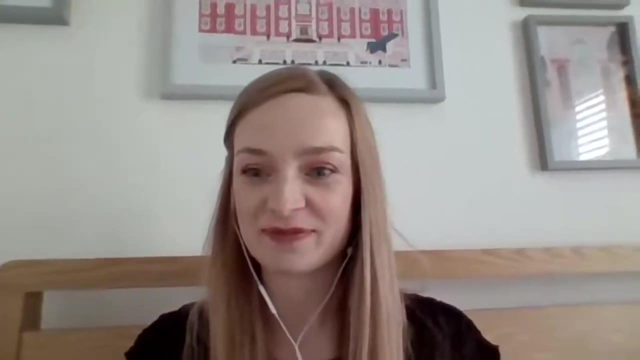 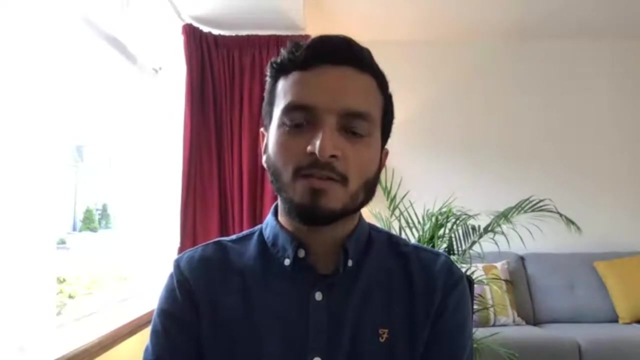 Sorry about that. Our next one is: can more diverse plant communities result in more carbon sequestration? Yes, there is. there is plenty of evidence from biodiversity experiments on that. Some of some of the big experiments going on in Germany or in the US show that pretty. well, Diverse plant communities give give diverse root exudates or root litter, So there is also a diverse substrate available to the diverse Community in such environments. So, yes, they do help carbon sequestration. I actually have a paper that was published in 2016, which shows just that. 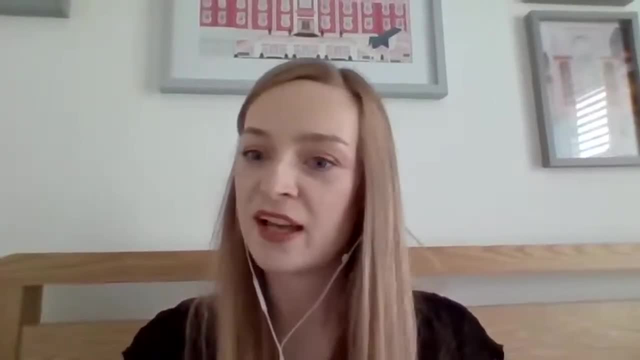 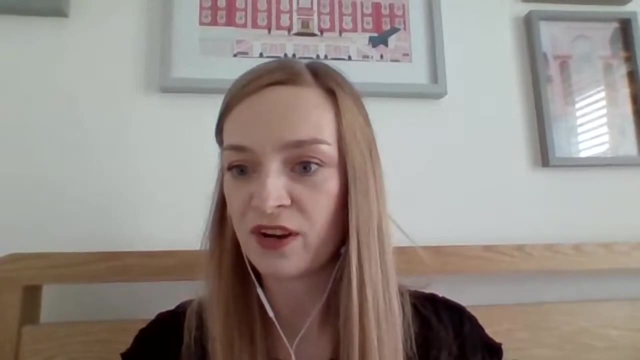 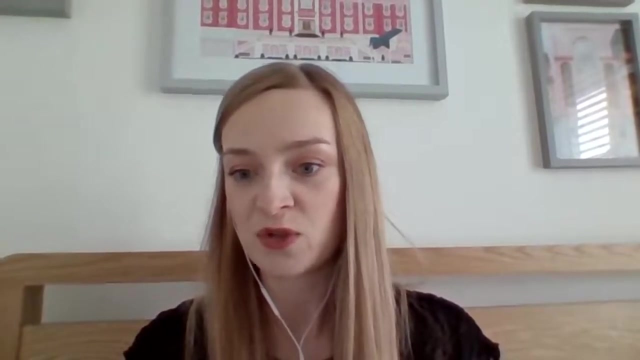 And our next one is from here, Darren, who says thank you for the presentation. Thinking on strategies for CO2 reduction, Do you know if there is any international project Or initiative aimed at the use of degraded soils for CO2 sequestration? 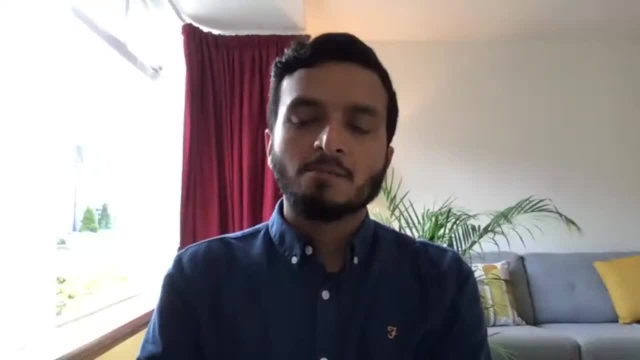 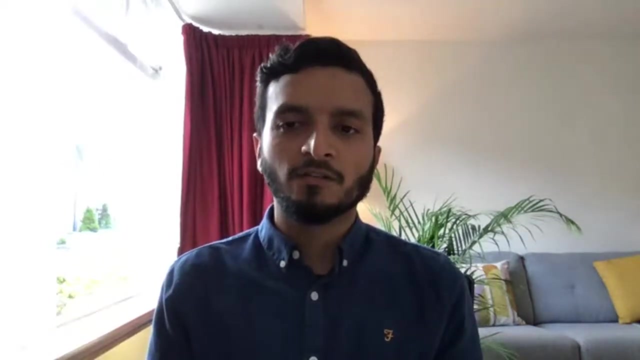 Yes, the classical example is the French initiative of four per mil. If you, if you look up four per mil initiative, that will link you to the, to the project that's actually trying to increase carbon sequestration in some of our projects. So that's the French initiative of four per mil. 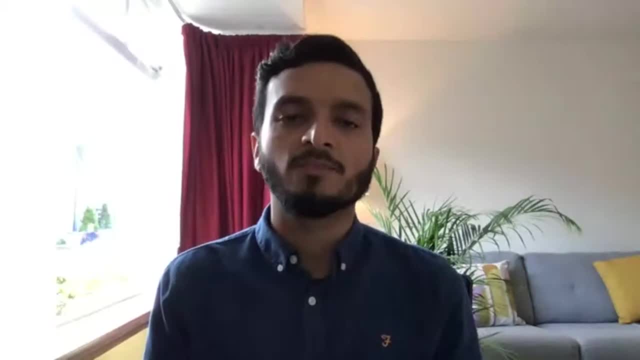 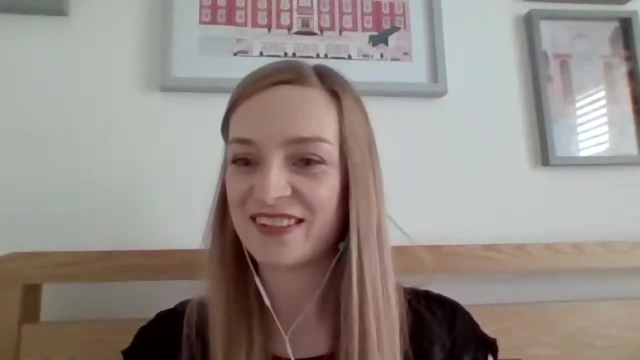 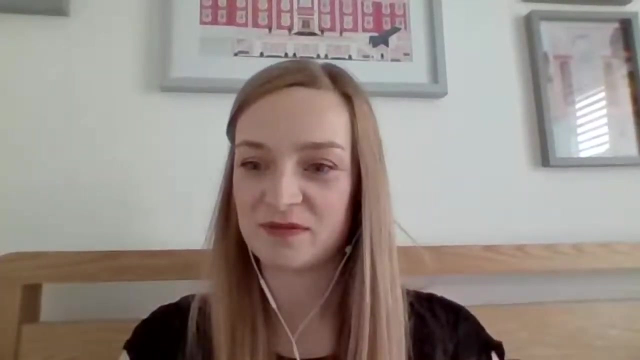 That's actually trying to increase carbon sequestration in some of our projects, In some of the most degraded soils. And are there any more questions? Just give it a minute or two. Yeah, I just want to add that EU is also trying to really ramp up. 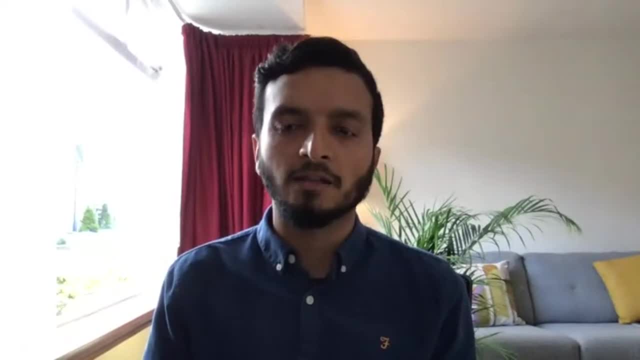 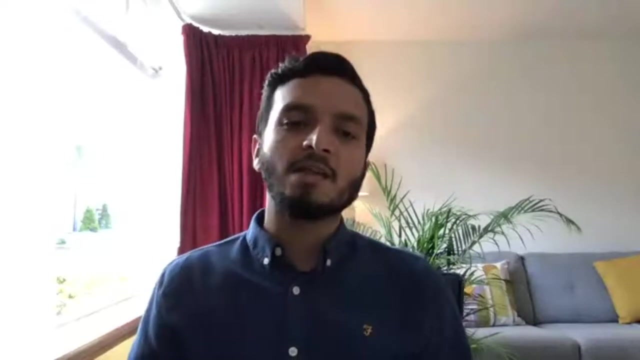 They are funding on soil health and carbon sequestration. So it's not It's not yet funded, but some of the newer funding programs, like the horizon europe, is, for example, trying to target research, that's that will be primarily aimed at improving soil health, carbon sequestration. 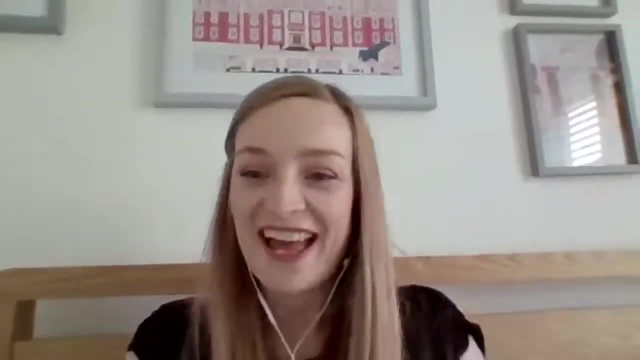 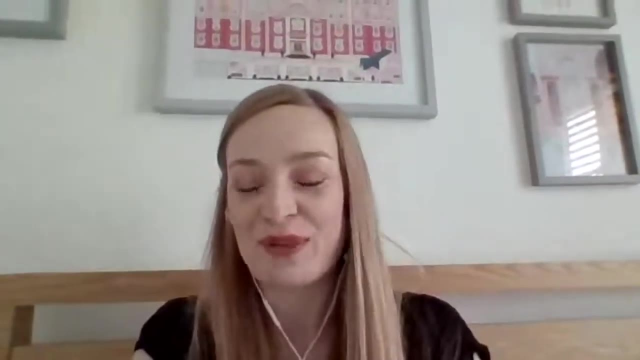 cool. our next one is actually a question that i can answer. um, so after the presentation is actually okay, nicole's just typed it, we're recording this, so we will to share that with you if you missed some of it. um, and the next question is from mary. uh, for best carbon. 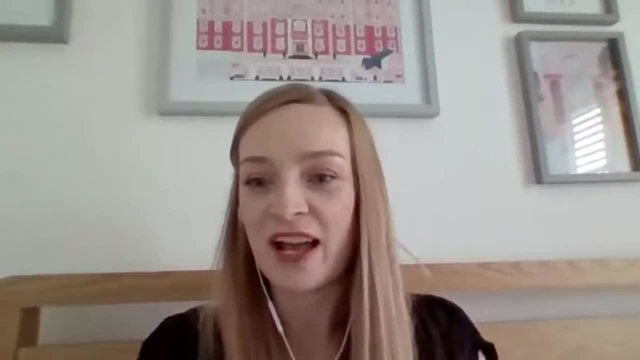 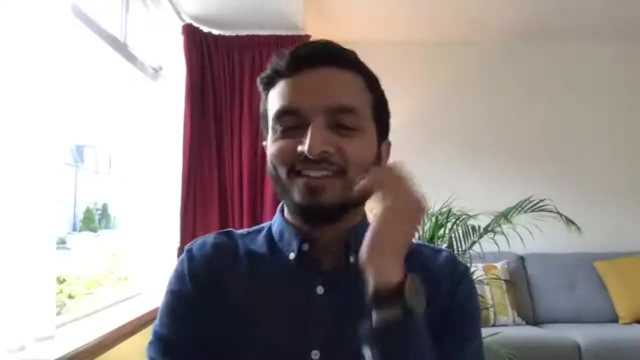 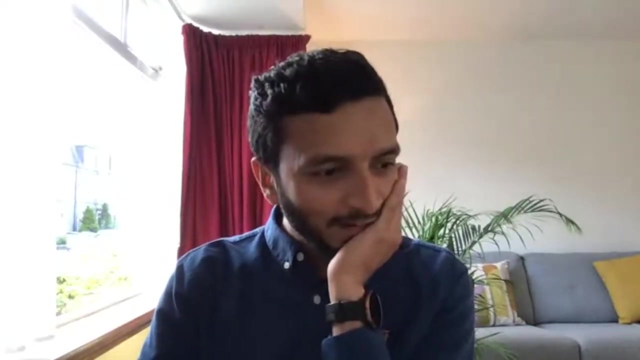 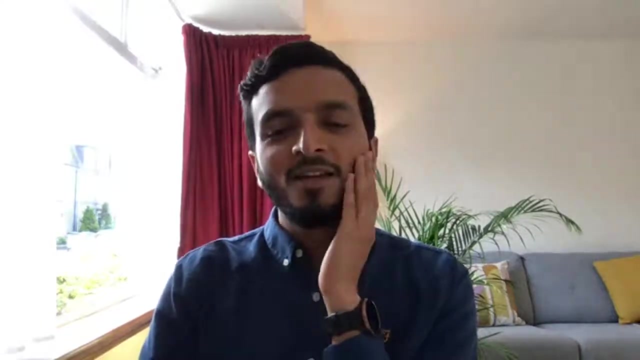 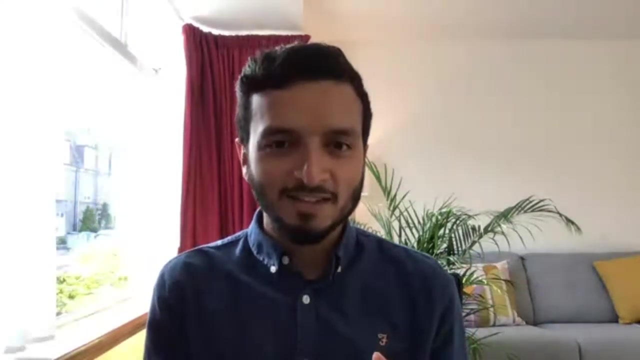 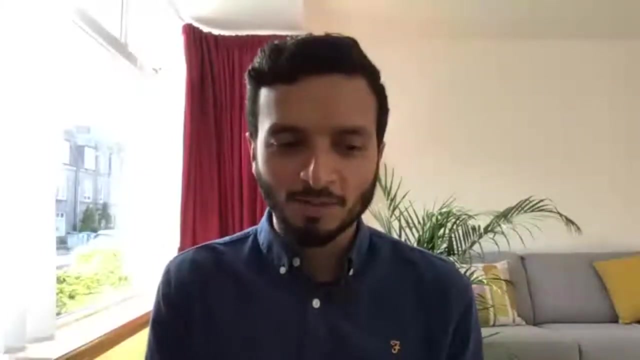 sequestration. how often should i mow my lawn? i have left it unload, i i'm not very sure about this. yeah, i didn't this. this would be a great experiment actually, um. so leaving it unmown um will feed root, exudates um and when it's senesis it will give up. um give up carbon better, and there's some indication from. 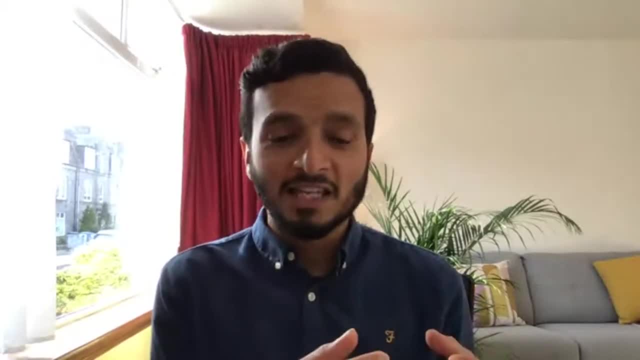 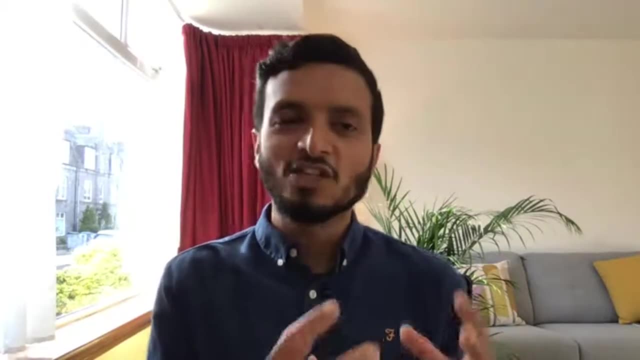 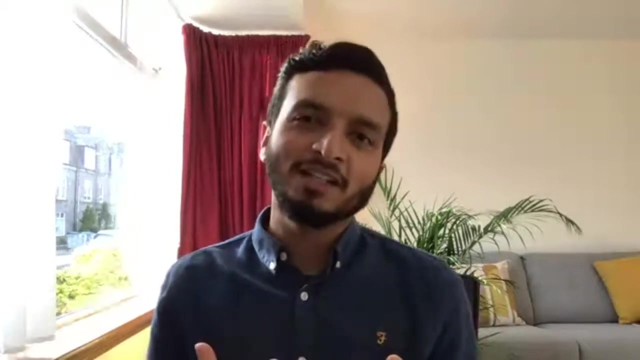 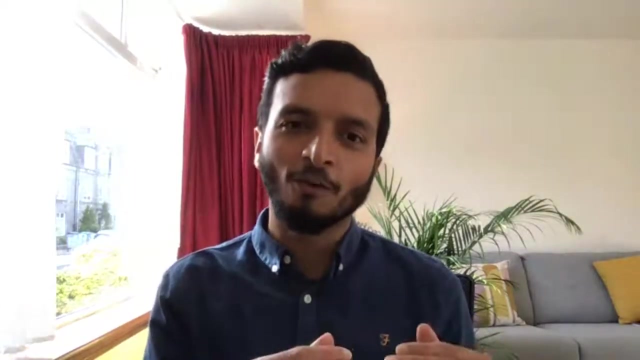 some of the research um that grazing actually improves root exudation because um the grass sort of dies and regenerates, so then it can um keep growing roots. but then there's also other indication that when you cut the grass um you're actually stopping that flow. so i'm not really sure. based on some 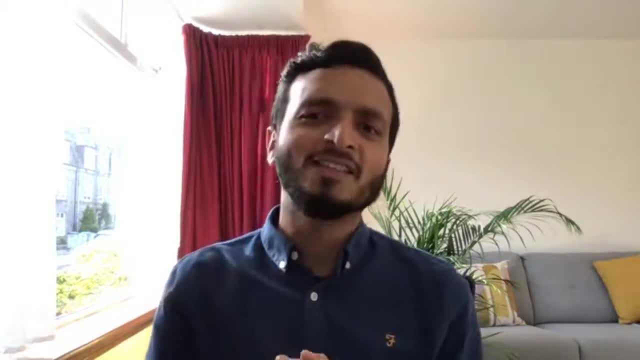 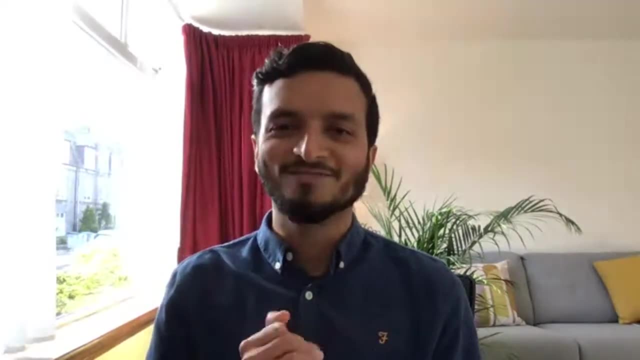 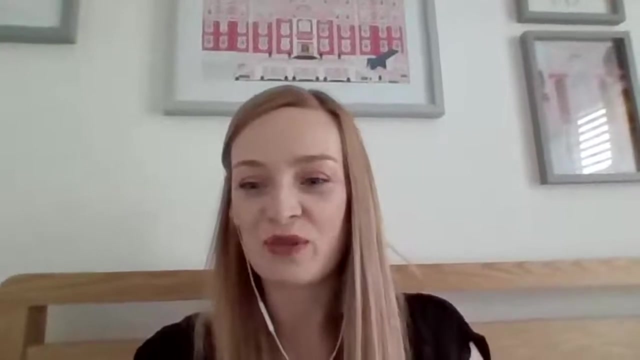 of the scientific evidence that happens. but i think this will be a great experiment, particularly from the science communication point of view. so thanks, mary. and there's another question, um, is there a potential for research to look at some of the urban development sites and qualify the carbon loss? 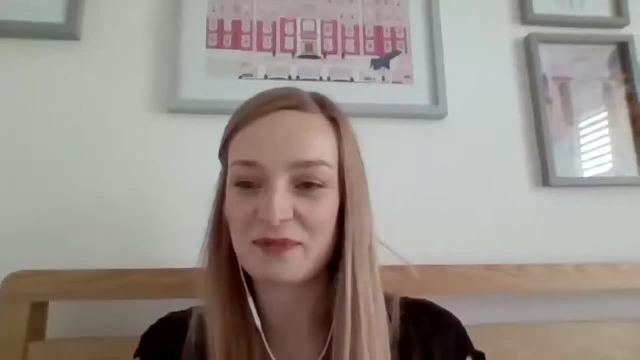 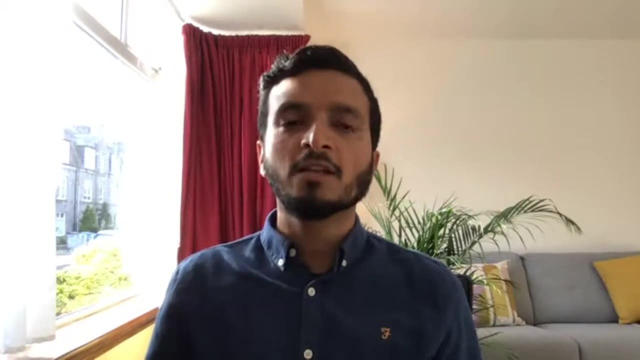 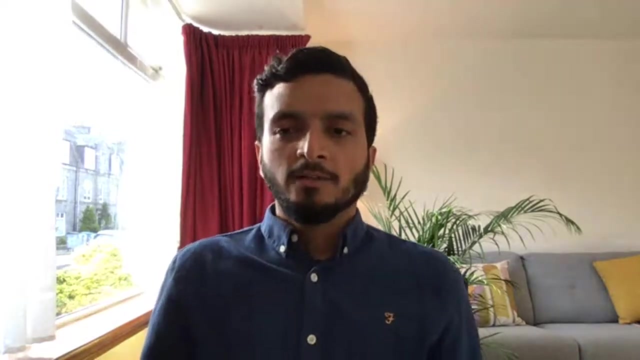 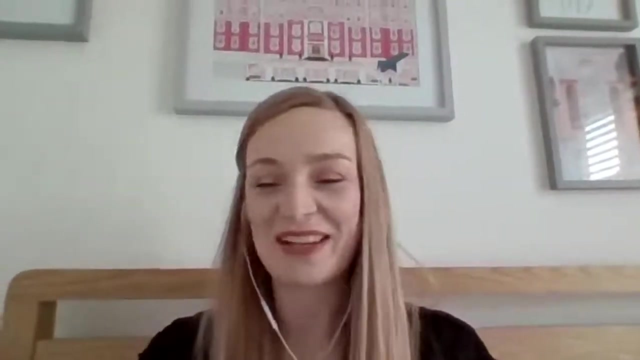 oh yeah, quantify, sorry. yes, yeah, this is definitely an area where not much research has been done, so this is definitely a place where there is plenty of potential research and there's a big potential for some of the work to be done here. i will recommend that you give it a shot. 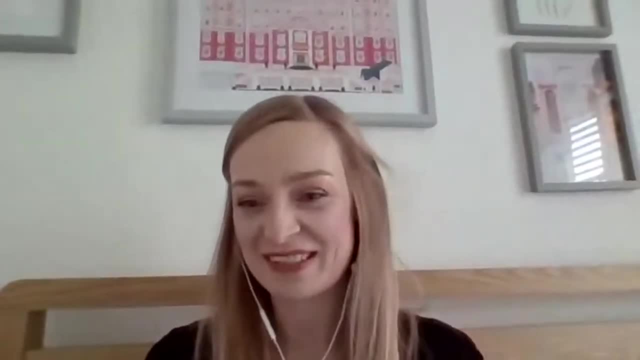 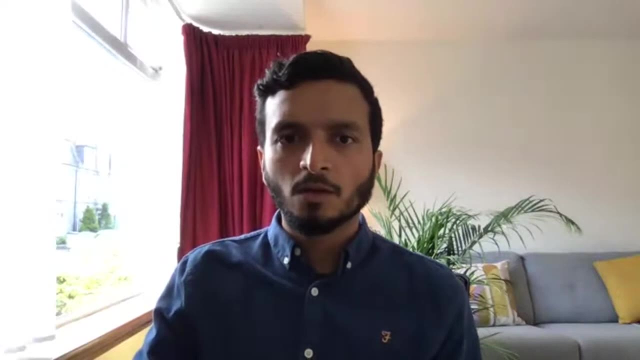 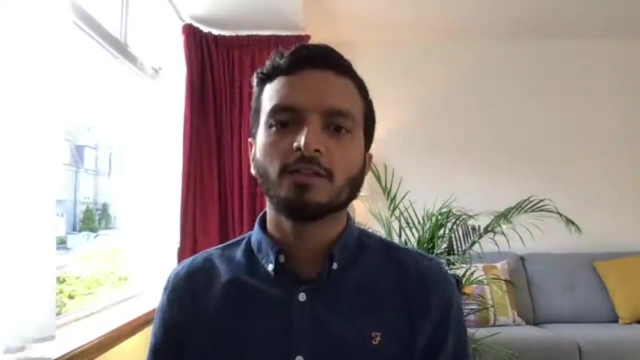 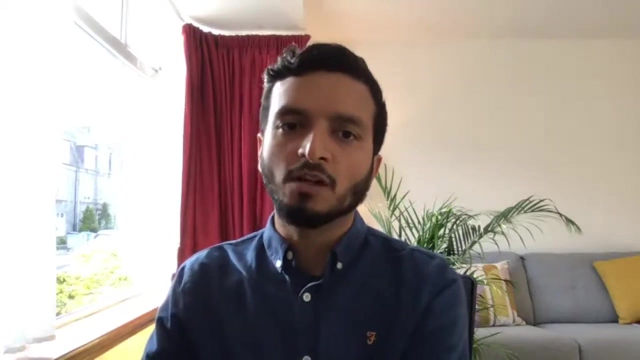 great. i'll again give it a minute because every time i think i've said: is there any more questions? there has been. so i'll just wait and see if anyone types. so i just shared the link to the full per mil initiative which is trying to um, like i said, mostly driven by the french government. 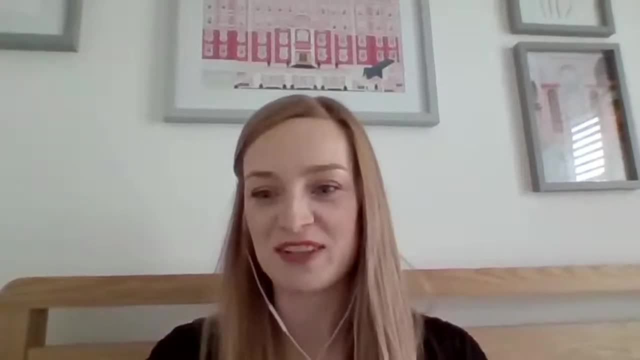 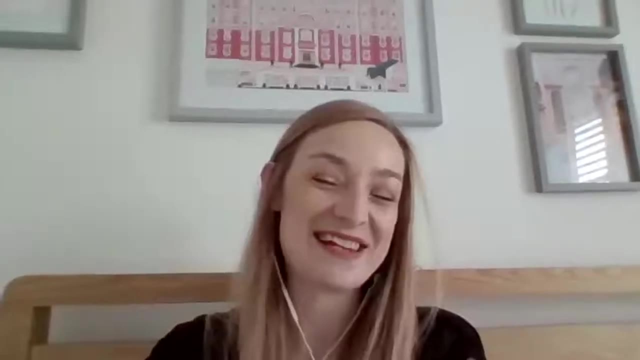 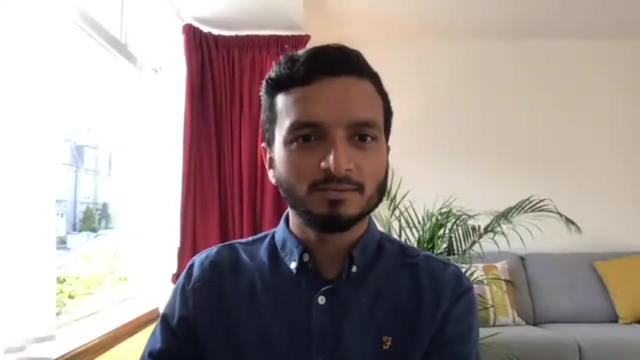 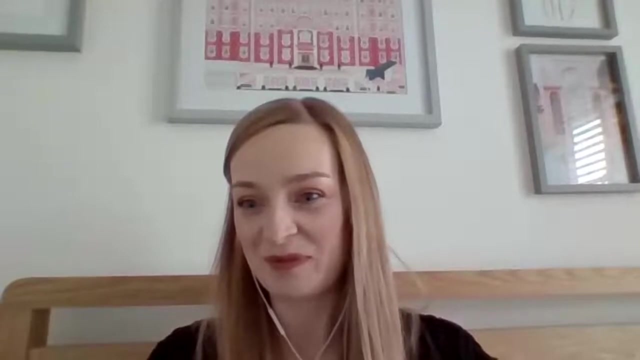 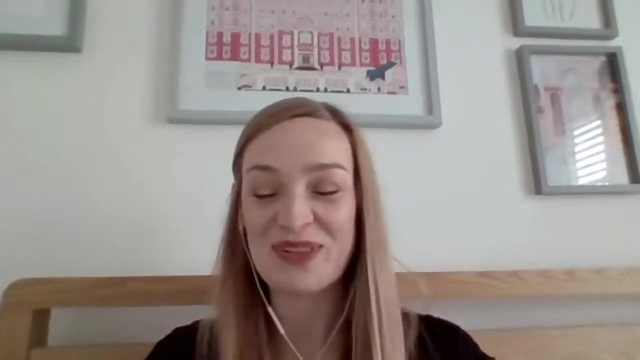 and aftabs just asked: would you be happy to be involved in such a project? yes, just need to get that set up now, okay, um, if there are any further questions, obviously just type them. um, aftabs just said: thanks, i will contact you then. um, i will leave that as a discussion between the two of you. 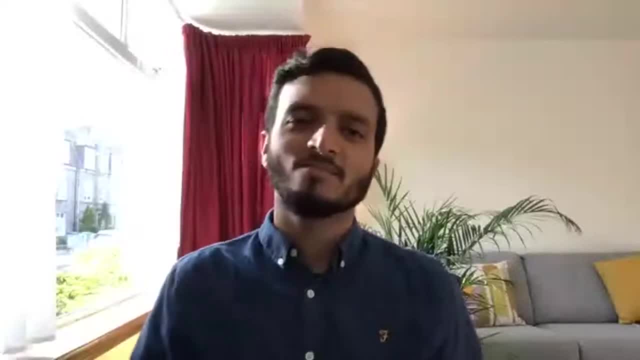 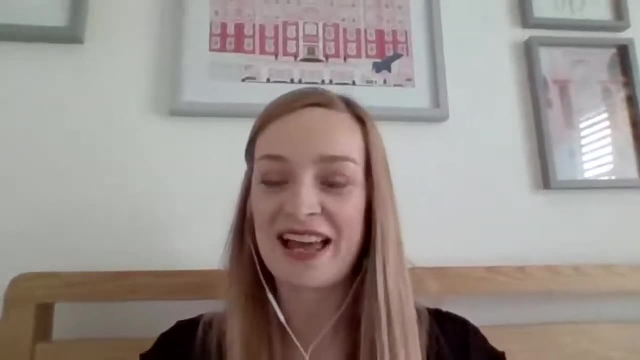 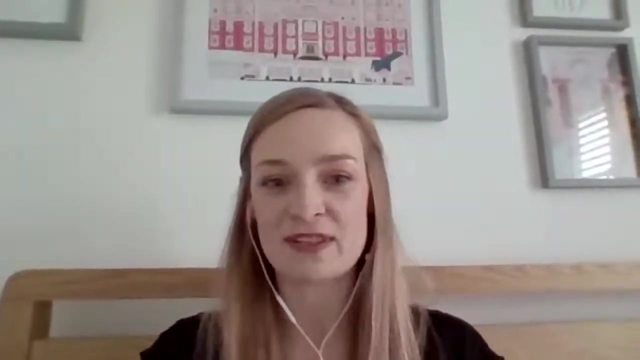 um, but yeah, thank you so much for presenting today and for answering all those questions. apologies if my pronunciation of things were not perfect. um, and i think you can kind of see there's some requests for contact details and obviously we've shared the recording. there's some information on that and if the email address 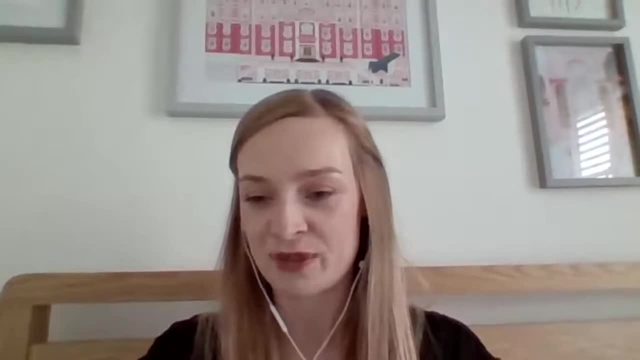 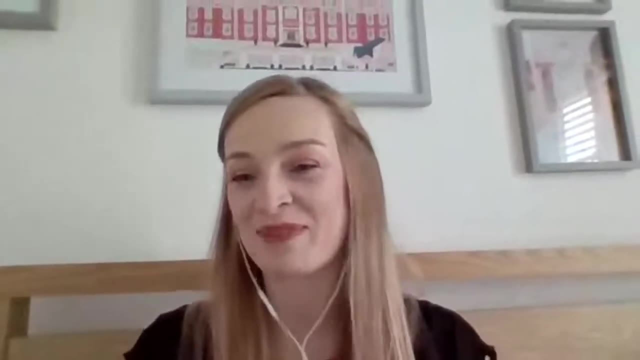 is there, then i can share that in the email that we'll send to everyone afterwards. um, but yeah. so thank you to ashish, and thank you to everyone for joining us today, and i especially think i recognize a couple of names who were here with us this morning. so, and thanks to everyone. 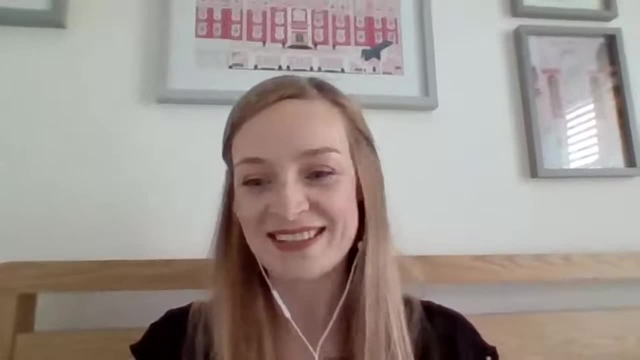 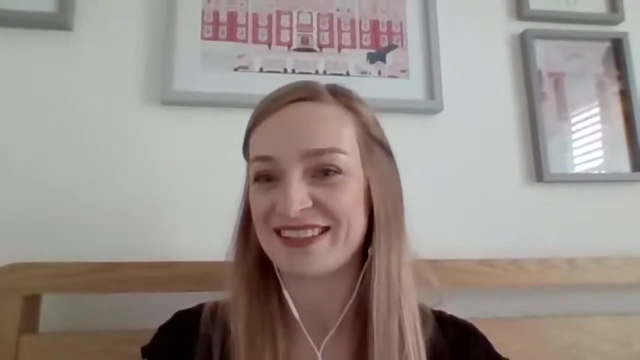 who's joined us for both sessions as well, and, yes, thank you very much for having me. no, no problem. um so yeah, i hope everyone enjoys their evening and has a great weekend when it comes.